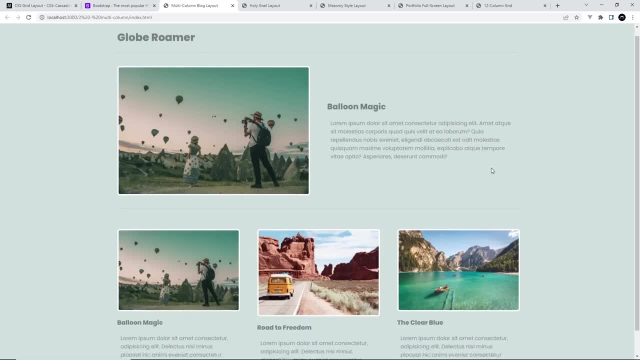 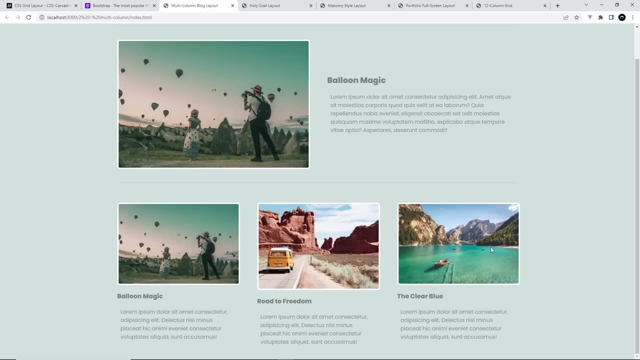 can see, we've got one big featured article at the top of the page, spanning the whole width of the site, and then, underneath that, we've got three columns of equal width With an article in each one, and it's CSS Grid that's allowed us to make these three columns. 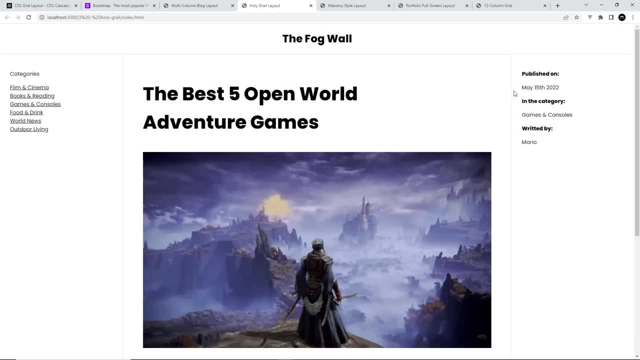 really easily. The next layout looks something like this: We've got a header at the top of the page, then underneath that, a sidebar- the main content- and another sidebar on the right. So these are all three columns of content, of different widths this time and at the bottom. 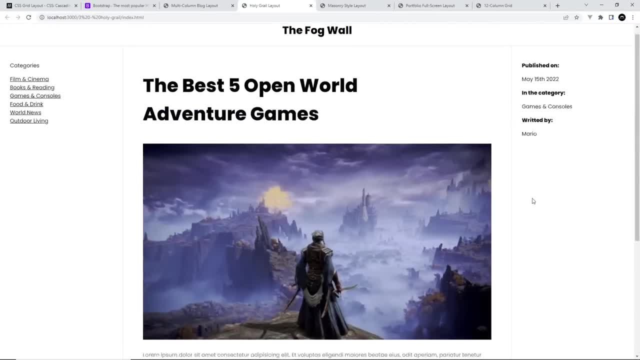 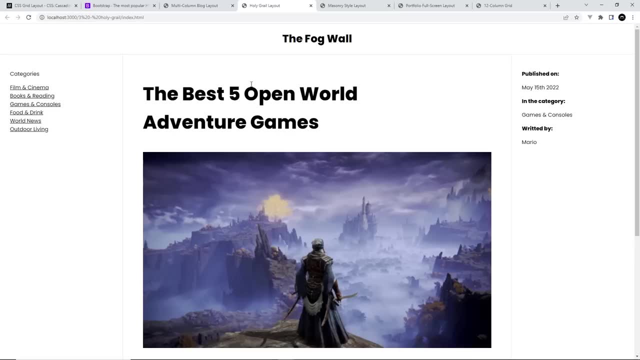 we've got a footer as well, and this particular layout is commonly known as the holy grail layout, because it's kind of like a go-to staple layout that works for a lot of different sites. So if you were to have a quick google of holy grail layouts, then you're 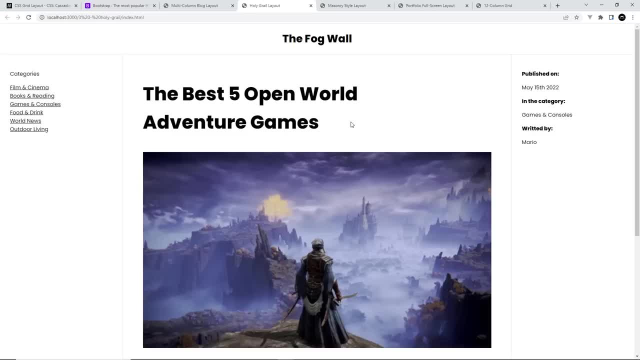 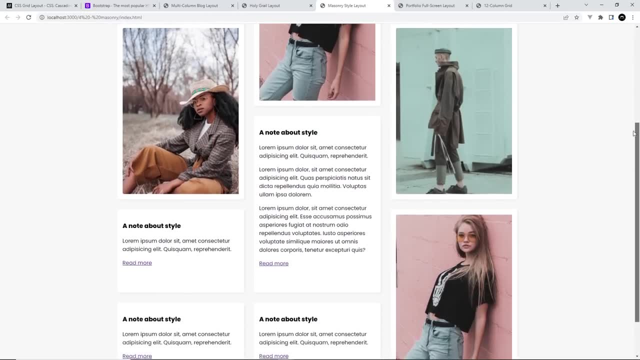 going to see a whole bunch of layout designs that look something like this. Anyway, the next one is a masonry style layout, which is basically a grid of elements that all have different heights, and technically this ain't going to be 100% pure masonry, because the height of each element is 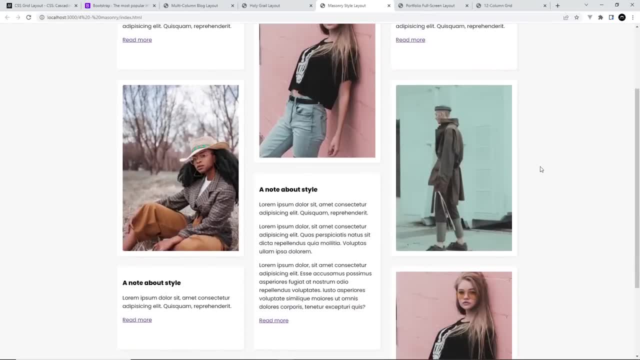 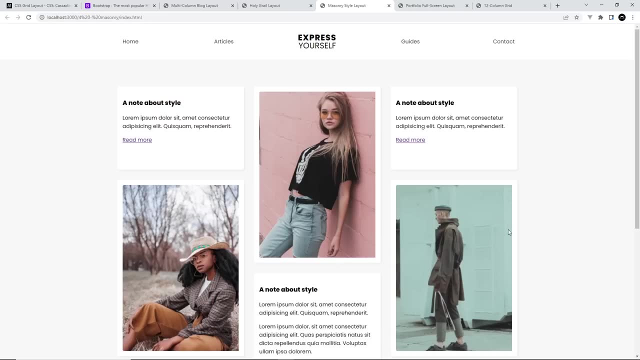 not going to be dictated by the content. Instead, we're going to give classes to elements to change how many rows each element should take up in terms of their height, But it still looks like a pretty nice version of a masonry grid, and after that we're going to create 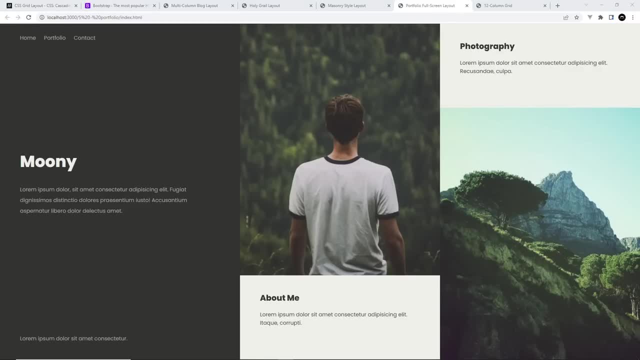 this next layout, and this is going to be a full width layout with three columns of different widths, but also in each column we're going to have nested grids to lay out the content vertically, which is pretty cool, and the inspiration for this design actually came from something I saw. 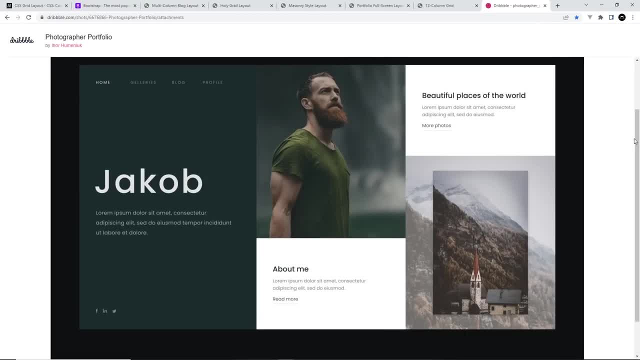 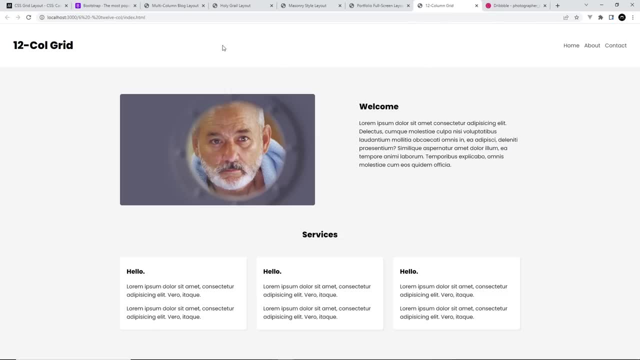 on dribble this thing right here and I've just changed some of the images and the text and whatnot. And then, finally, I'm going to show you how to make a 12 column grid system, and then you can use that to spread content onto it however you wish, and this: 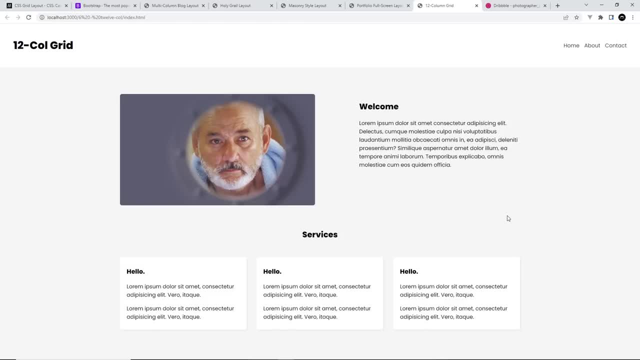 is really cool for when you've got quite tall pages with a lot of content that's displayed in different ways, like this, or just when you want to quickly prototype a design for someone. So that's a quick preview of the layouts that we're going to make. but first off, like I said, 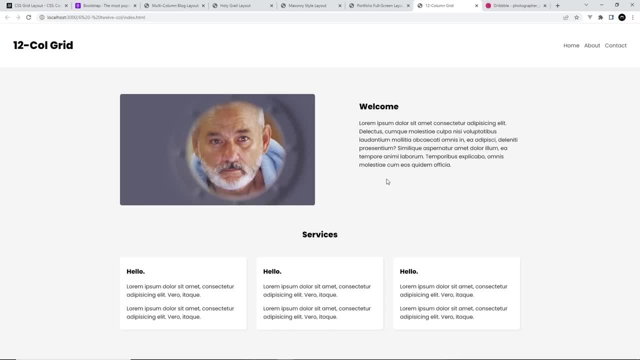 before. I want to do a quick overview of the basics of CSS grid, just to bring everyone up to speed and on the same page. But feel free to skip this if you already are comfortable with CSS grid and you just want to dive in to make those layouts. 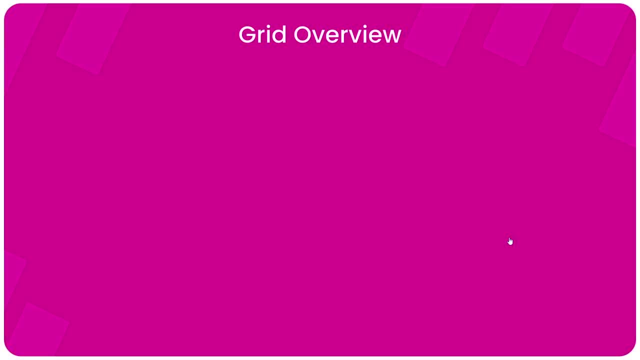 So, then, CSS grid, as the name implies, allows us to display content in grids on a web page, and those grids are made up of columns and rows. Now, it's totally up to you how many columns and rows you want the grid to have. We could have three columns, or six, or eight, or more, etc. and as 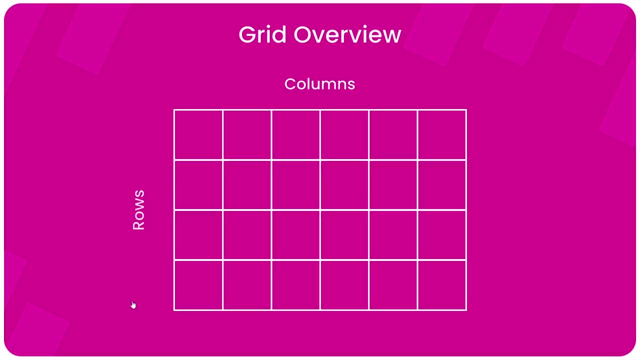 for rows. we could have two or three or four or as many as you wanted, and then we can just choose how many columns we want to display on the grid by specifying how many columns of width it should take up and how many rows it should take up as well. For example, this element right here takes: 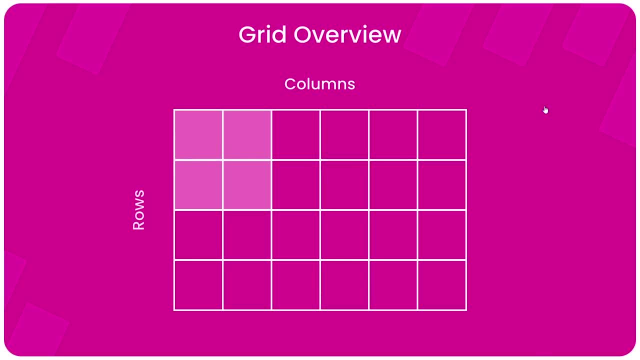 up two columns in width and it spans two rows in height as well, and we can also choose the position of the content on the grid, too, manually. So if I wanted to, I could place this next element over on the right of the grid in the fourth row. It's entirely down to you where you want to place your. 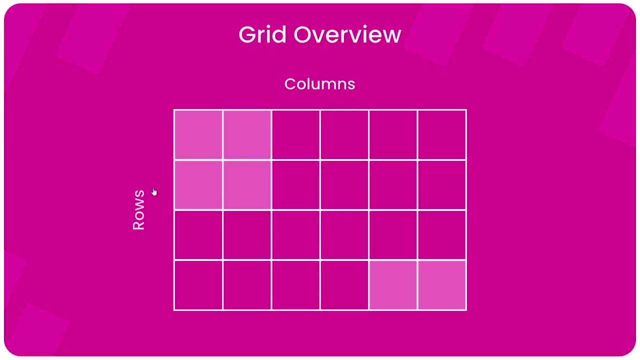 content in the grid when you've created it. So we've got rows, columns, and the elements placed on the grid are typically called grid items. Another bit of terminology might come across is the word track, and a track is just another name for either a row or column. So 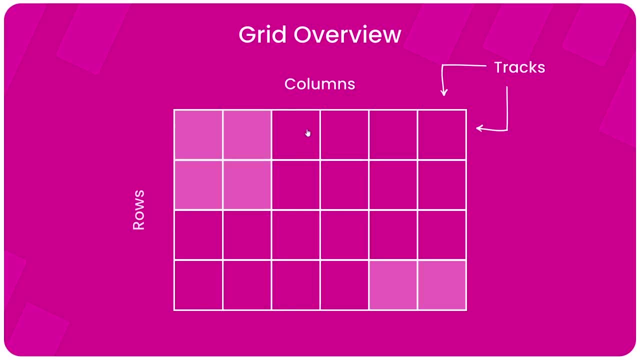 this first column would be a track, the third column would be a track, the second row would be a track, etc. Every single row is a track and every single column is a track. We also call the lines between the rows and columns or tracks, grid lines. So 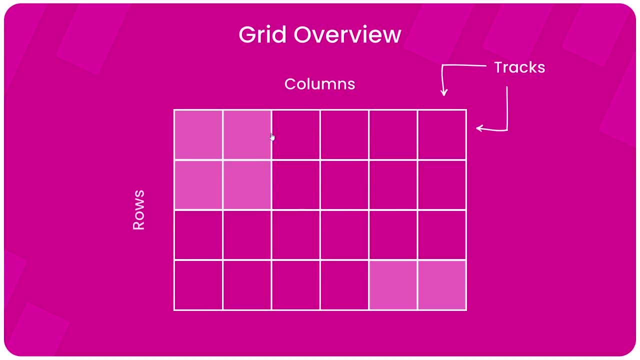 we've got these vertical grid lines between the columns and we also have horizontal grid lines between the rows. Now these grid lines have numbers associated with them. They start at one and increase by one all the way to the end of the grid, and they do this in both directions. 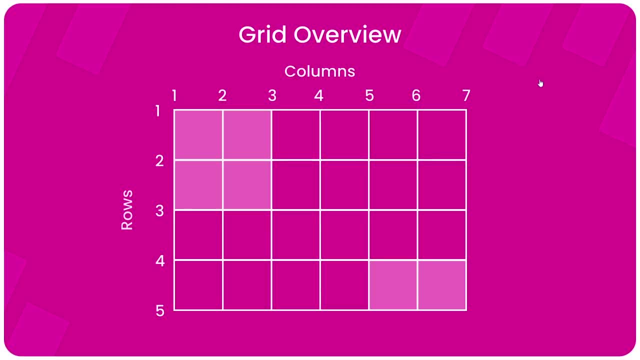 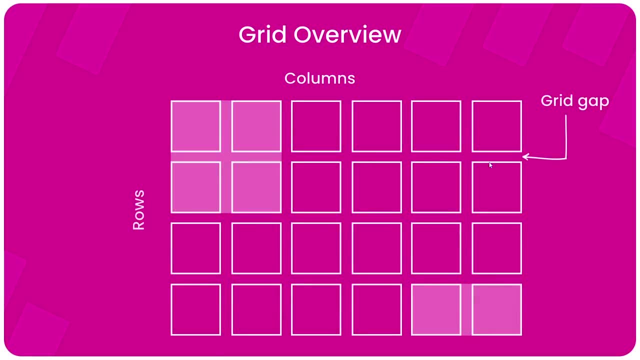 and these line numbers are important because we're going to use those to specify exactly where we want to place our content later. And one more thing: we can have gaps between the columns or the rows or both, and these are typically called either gutters or grid gaps, and they're a way to 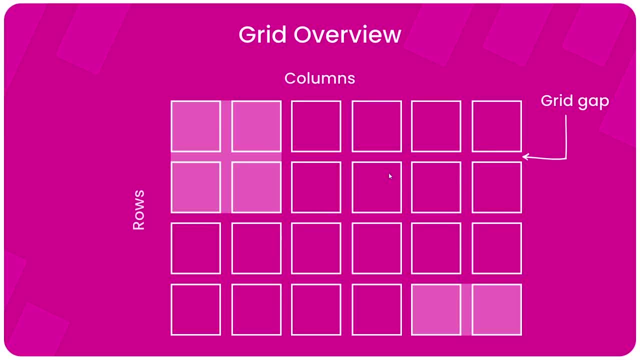 kind of space content out on the grid, so that each grid item isn't squashed up to the next one. Okay, so that's a bit of basic theory and terminology. Next up we'll see this in action and go over some of the basic grid CSS properties. Now, before we dive into the code, 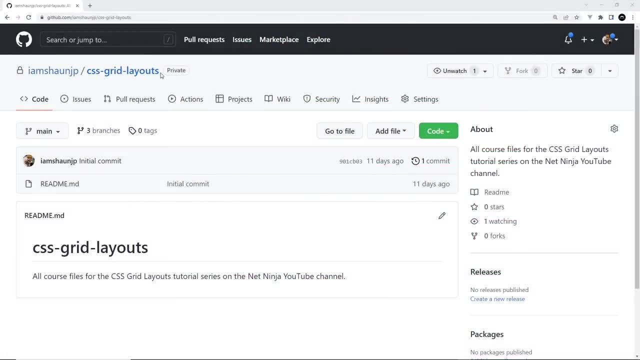 I just wanted to let you know that I've uploaded all the course files to this GitHub repo right here- and I'll leave a link to this down below the video- And this repo's got just two branches. The first branch is the starter files branch, which contains all the starter files. 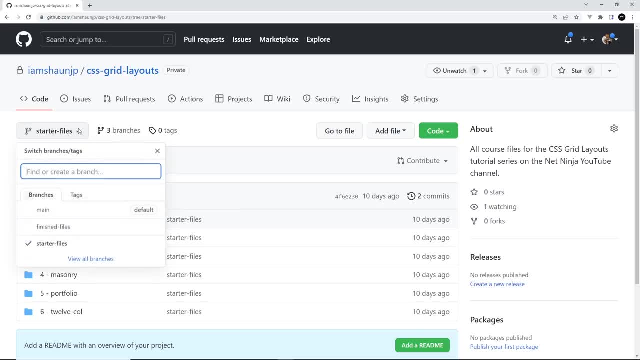 and code for the different projects that we're going to be making. And the second branch is the final files branch, which contains all of the final code for the projects. So you can select any of these branches up here and then you can download that branch in a zip folder by hitting 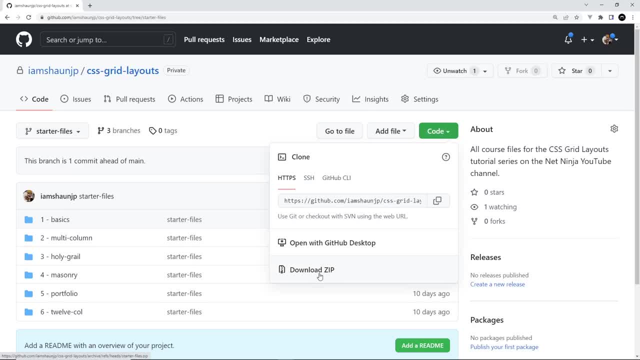 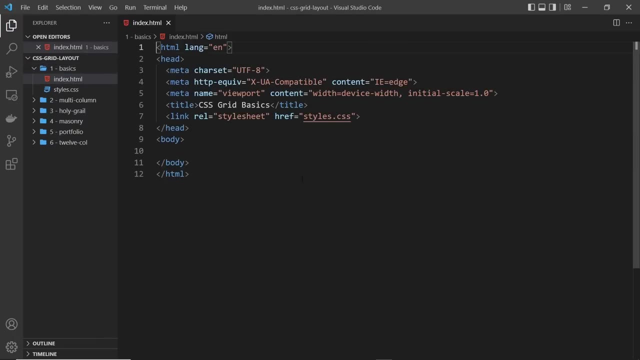 the green code button and then downloading the zip folder. So in this lesson we'll be working with the basics folder and then later on we'll be working through these other folders as well. So then I'm inside the basics folder and to start with we've got an html page- pretty empty- and that's linked up to a CSS file called. 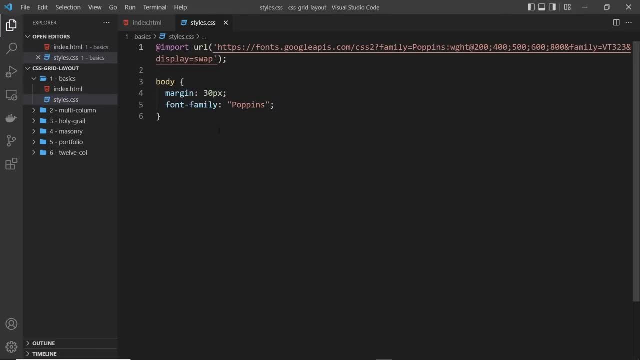 stylescss, and inside there is just a single body selector and a google font that we load in as well, called poppins. So let's go back to the html page and start making a grid and placing items onto the grid. So the first thing we need to do is make some kind of grid container. This can be any element. 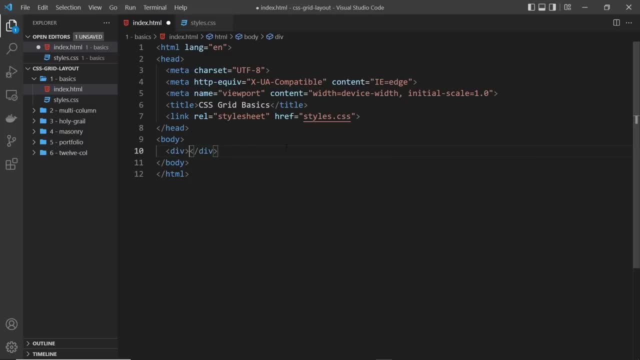 but I'm going to use a div tag And anytime you're going to use a div tag, you're going to want to make sure that you're going to use CSS grids. You always need a grid container and that grid container is essentially just going. 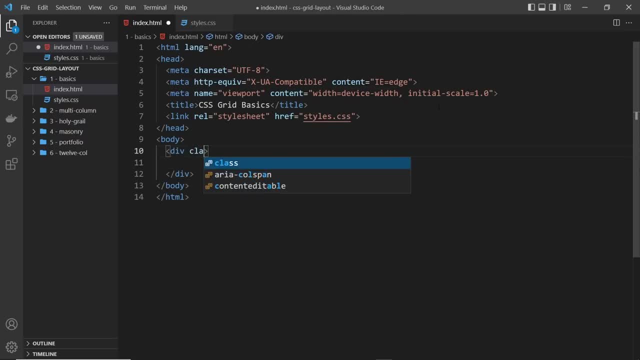 to act as the grid itself. I'm also going to give this a class of grid hyphen container so that we can style it later on as a grid. but you can call this class whatever you want, it really doesn't matter, And on its own in the html it's not a grid, it's just a div tag. it's in the CSS that we actually 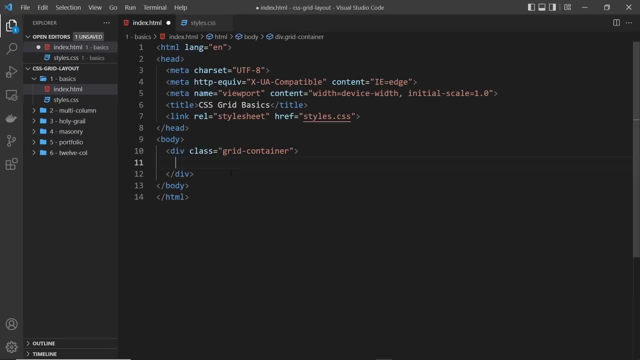 make it grid later on. So the next thing we want to do is make some grid items So content that we want to place on the grid, and these elements just need to be nested inside this grid container element, and any element directly nested in here is considered a grid item, So these elements can. 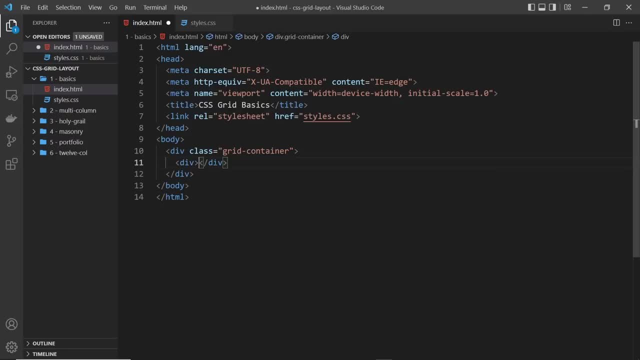 be anything: div tags, images, article tags, nav paragraph tags, etc. I'm just going to add in a few div tags to keep things simple, six in total, and I'm also going to place a little number in each one as well. So now we should have six grid items, right, and these are the things that we want to place on the grid. 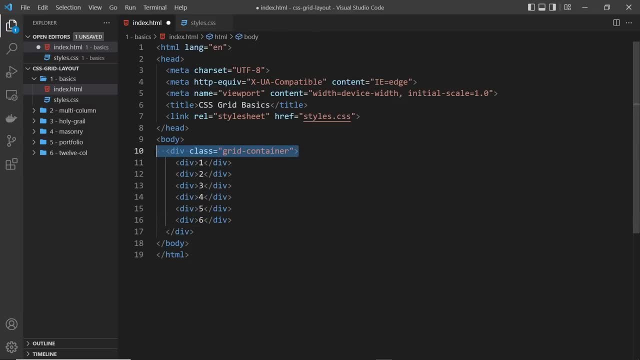 These are the things that are ultimately going to get displayed on the grid, and we can manually position them on the grid later as well. All right, all right now. the first thing I want to do before we style anything is just to open this up in a browser so that we can preview the work as we. 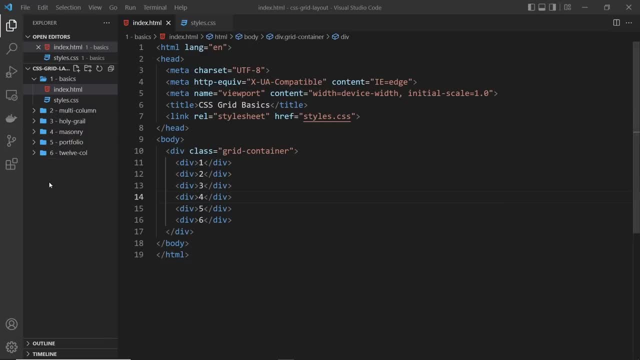 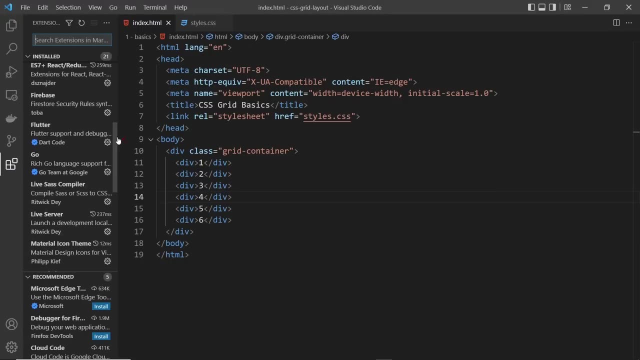 go forward, and to do that I'm using a package called live server. so to grab that in VS Code, just go to extensions and search for live server up here. I've already got it installed and it's this one right here, live server. and once you have that installed, 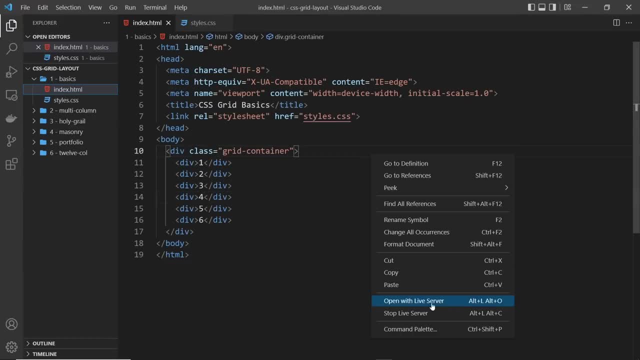 if you go to any HTML page and right click, you can open up with live server and that's going to spin up a local development server with live reload so that every time you make a change and save the file it's going to automatically refresh and show those changes in the browser. So let me open this. 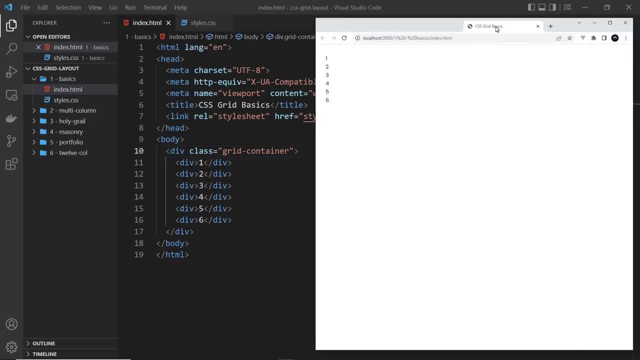 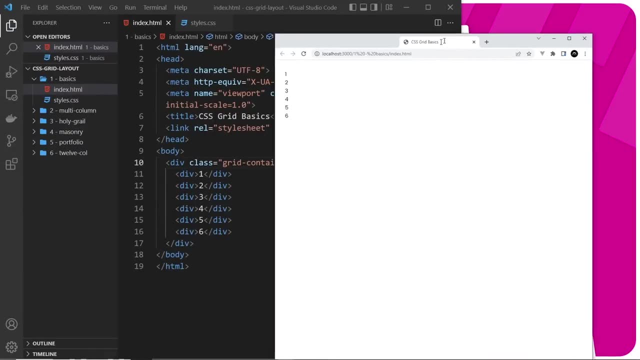 up and it should open up on a browser over here so we can see that. I'm just going to move it back over here so that I can do a bit of a split screen. let's make this half and then bring this over here as well, so we can see both at the same time. 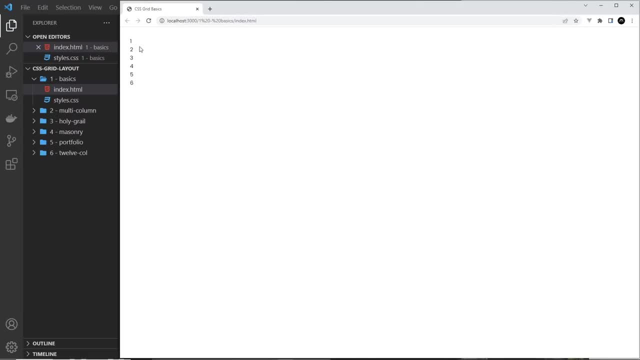 So that's how it looks at the minute. pretty crap, because we just have those six divs inside the grid container, but none of it is styled yet. so now what we need to do is style the grid itself so that all of these things right here become grid items and we can start to distribute them. 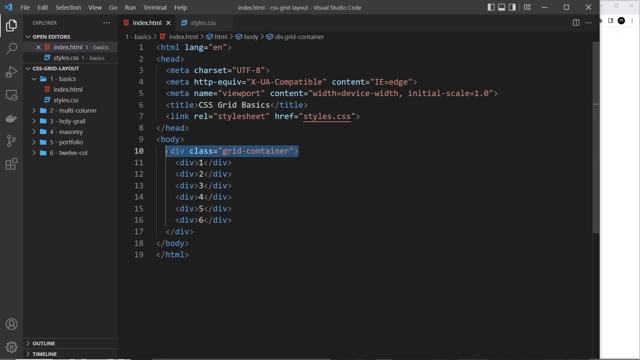 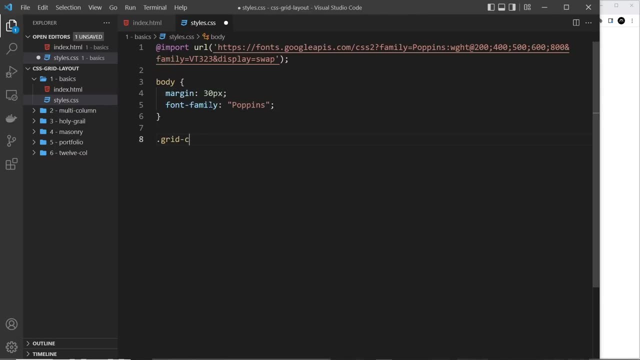 on the grid. So the first step is making this div right here an actual grid so we can use this class selector over in the CSS I'm going to say grid, hyphen, container and then in here, the first thing we're going to do is, in fact, before we do anything with grid, I'm going to set this to have a background. 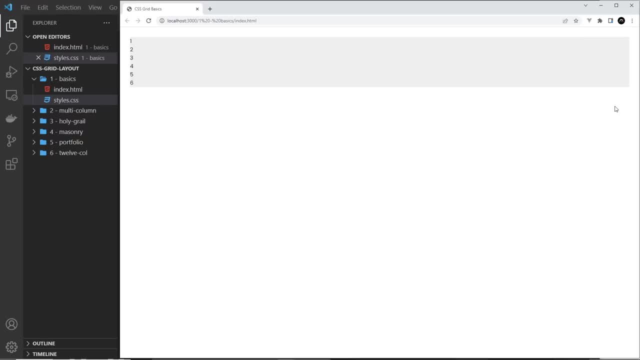 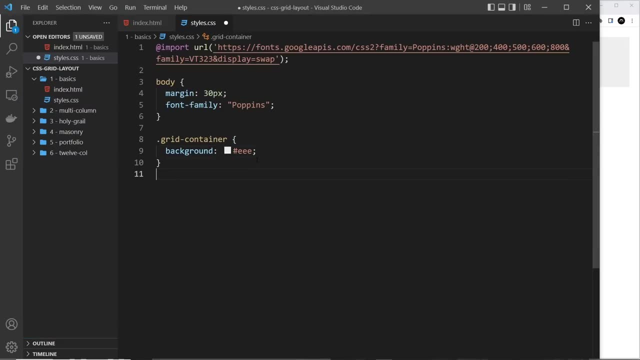 of ee, which is a light gray, just so that now we can see that on the page and we can see this thing here. this is the grid container, right, and in fact what we'll do is a similar thing for the grid items. so all of the divs inside here, we're going to colorize those as well. so let me say grid hyphen. 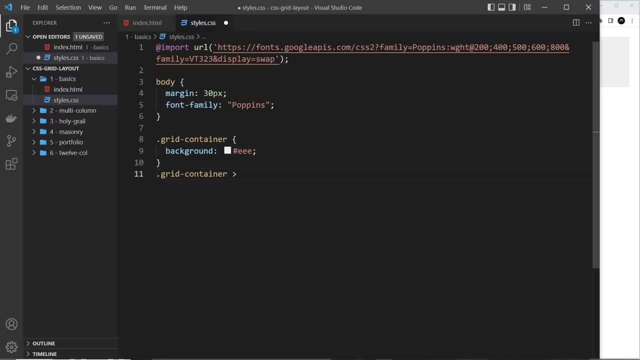 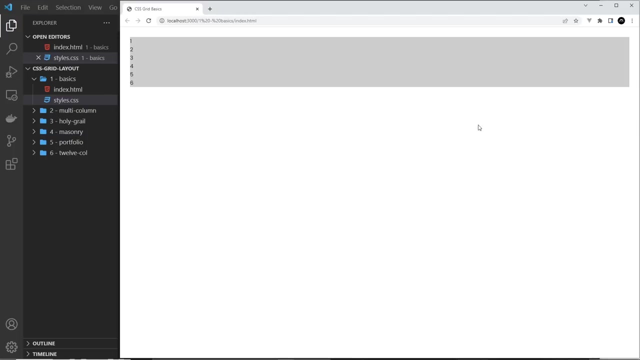 container. and then we want to do forward angle bracket and then div, to say any correct descendant which is a div is going to become a grid item, right. and we want to give those a background of ccc which is a slightly darker gray, so they stand out as well. so now we 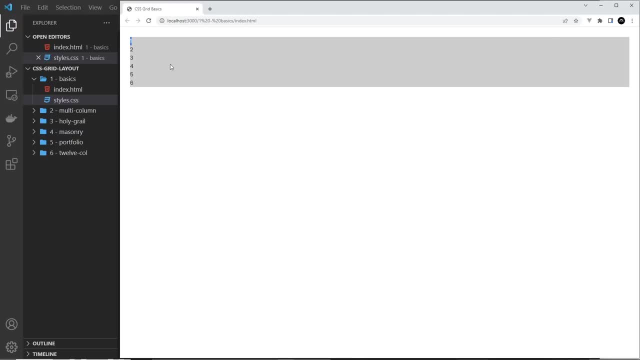 can see all of these, and they all stretch across the whole div, because, by default, divs are block level elements, and block level elements all take up 100 percent width of their parent element. okay, so we have all those colored as well. all right, so what I'd like to do now is come up to this grid. 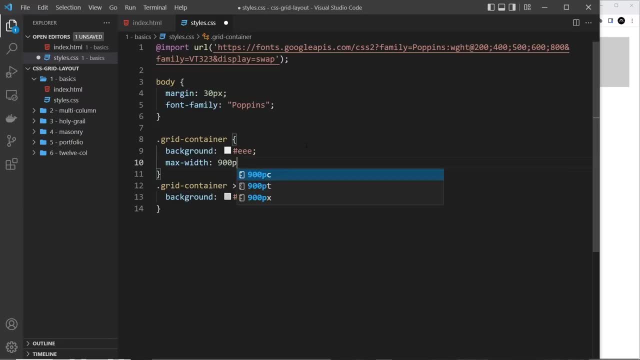 and I'm going to give this a max hyphen width of 900 pixels and also a margin of zero top and bottom and auto left and right, and what that's going to do is make this 900 pixels in width and sit it in the middle of the page because it's going to apply an auto margin of whatever is left. 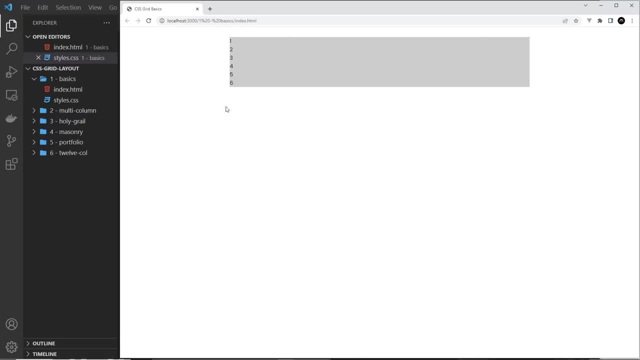 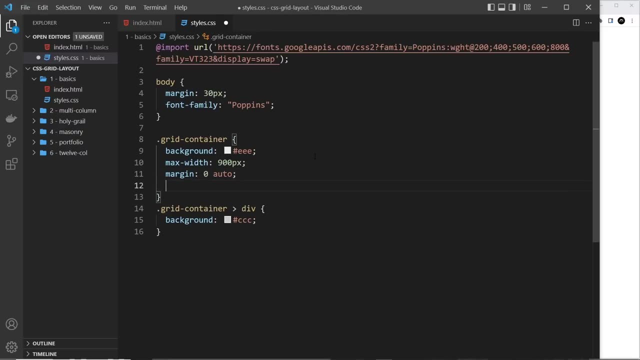 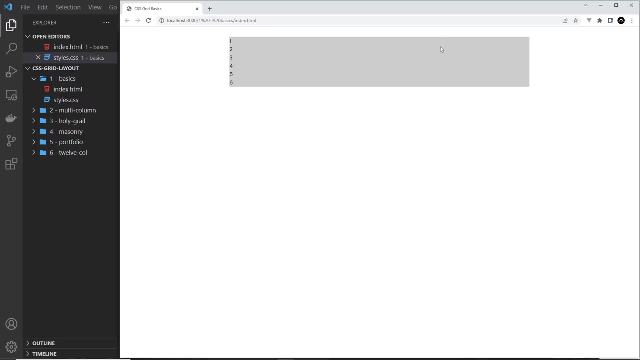 on the page to the left and right, so it should sit in the middle. so this is the grid container, but at the minute it's not actually a grid, it's just a div, and the way we create a grid is by just setting the width of the grid. so we can see the width of the grid. so we can see that. 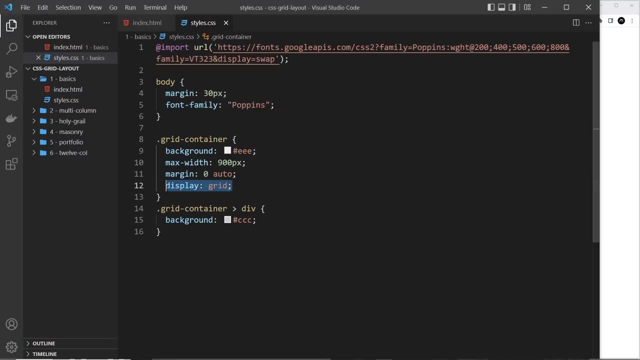 it's not a grid, right? so if I save this now and come over here, we can see that it looks exactly the same. so on its own, that's not really done much. all we've done is set it to be a grid, but what we need to do is define the columns in the grid: how many columns should we have and what. 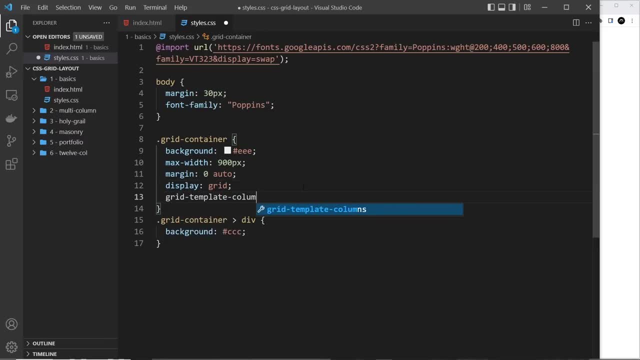 width, should those columns be. so the way we do that is by using a property called grid, hyphen, template, hyphen, columns, and then we can specify all the different columns that we're going to have and in our grid, and we can say 300 pixels, 300 pixels and 300 pixels for each column. so what this does. 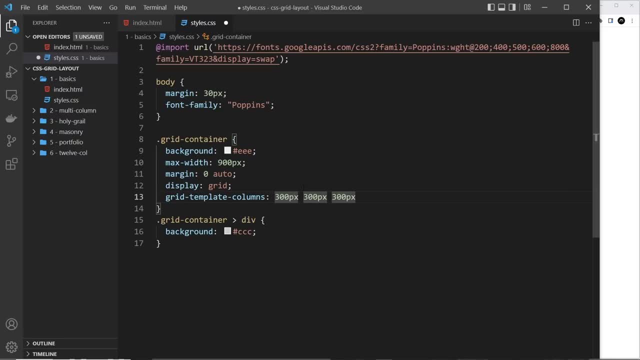 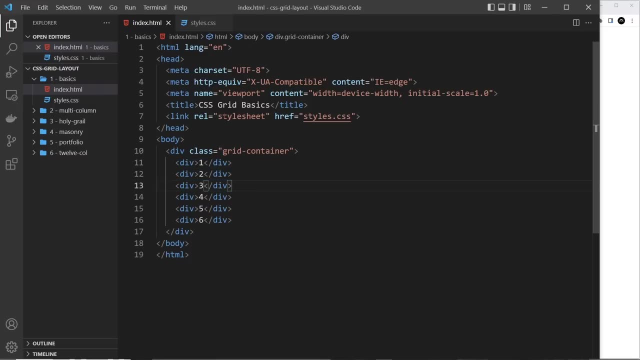 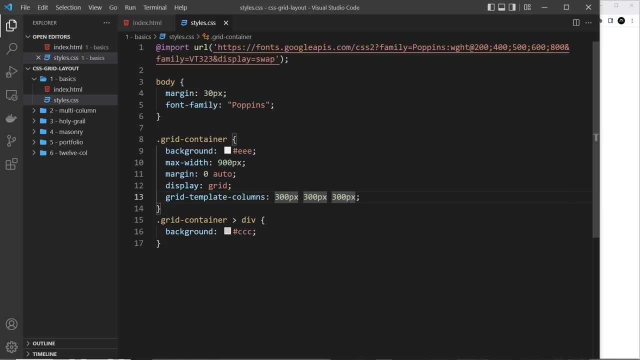 is create a grid with those three columns of 300 pixels each, and what it's going to do is automatically distribute each one of these at the minute into one of those columns. so, since this is 900 pixels in width in total and each one of these is 300 pixels in width, these columns they make up. 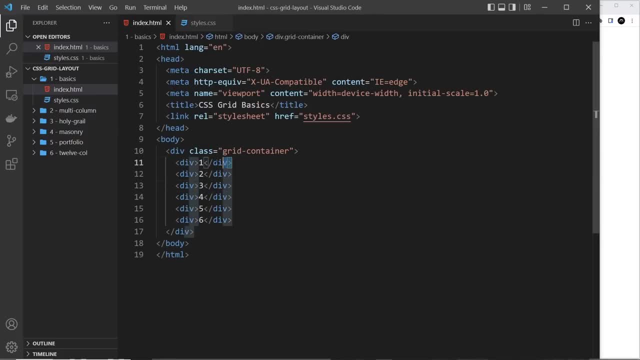 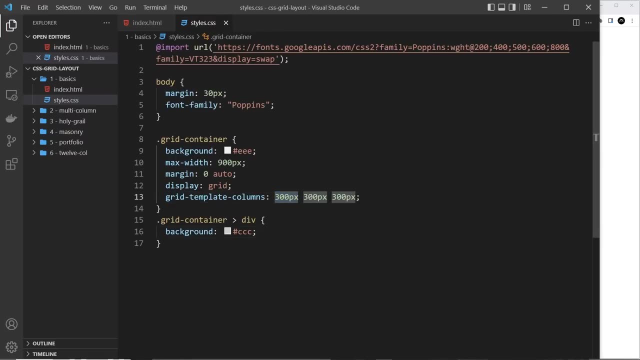 900 pixels, right. so what it means is the first, the second, the third, the fourth, the fifth, the sixth, the second and the third. they're all going to be on the first row inside this grid container and they're all going to be in one of these 300 pixel columns right here. so we should see the first three. 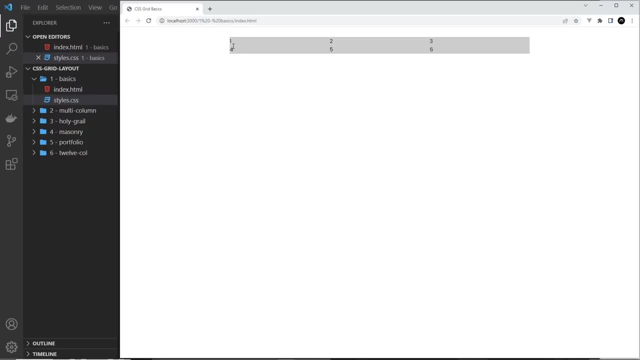 on the top row and the second three underneath. so if we check this out in the browser, we can see that one, two and three, four, five and six. let me just zoom in so we can see this a bit easier. all right, cool, now I'm also going to come to the grid items, these things down here, just so I can say: 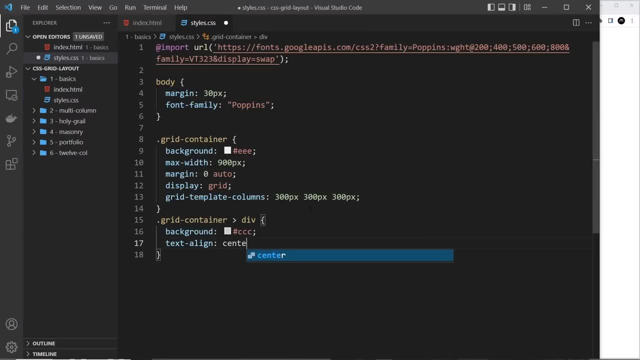 text hyphen align is going to be center, and then also the padding of each one is going to be 20 pixels, just to space them out a little bit inside, and we'll give each one a border as well, so we can see where each one starts and ends. 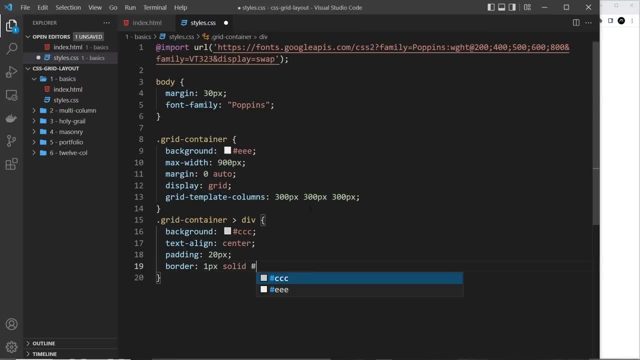 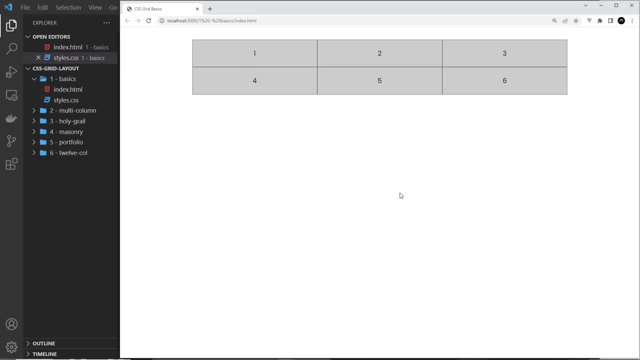 so border is going to be one pixel solid and it's going to be 777, which is a darkish gray, and if we check this out now, we can see each one of these grid items right here. so they're automatically being placed in each one of these columns. that's the default behavior. 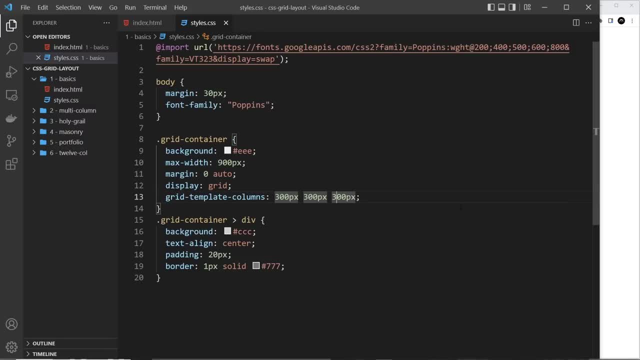 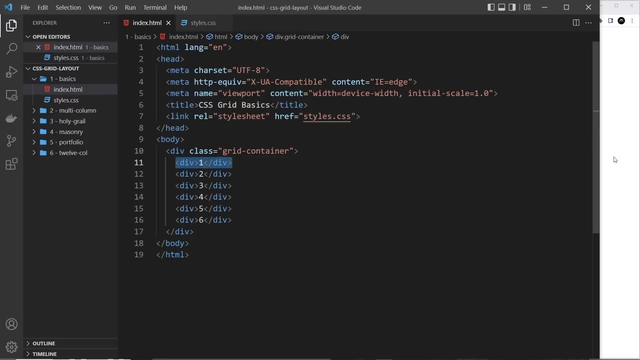 now we can override that- which we'll see later on- where we can manually assign different spaces in the grid to the items. for example, I could say something like this: first one is going to take up the first two columns in width, the second one is going to take up just one. 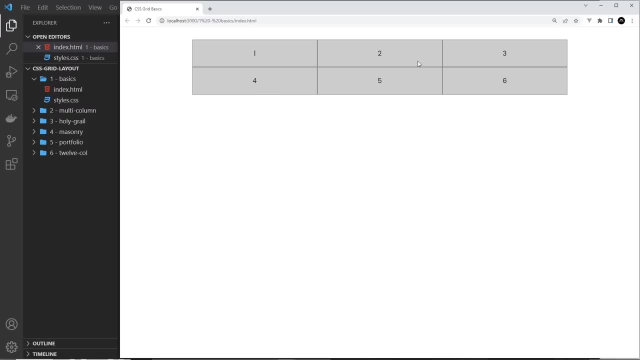 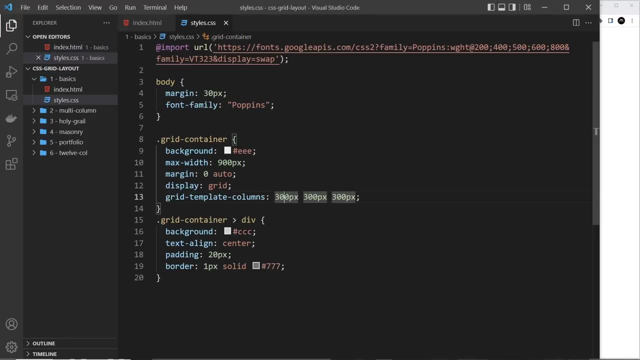 the third one is going to skip this section and start here and take up two, etc. so we can do things like that, but the default behavior is that each one of these is now sitting in a column automatically. all right now, imagine we wanted six columns instead. well, we could. 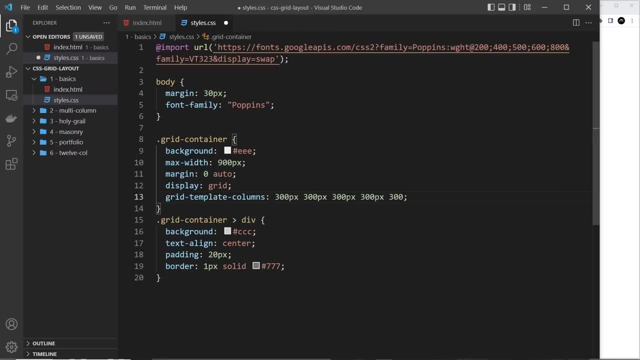 carry on and say 300 pixels, 300 pixels, and do this six times, but that's a waste of time. so what we could do instead is delete this, and we could use a function called repeat, and this takes in two arguments. the first argument is how many times we want to repeat something, so, for example, six. 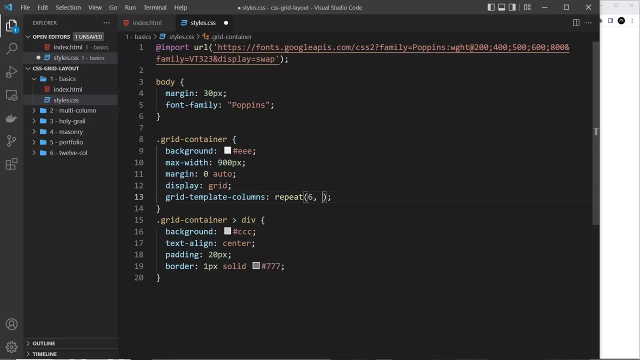 and the second argument is going to be the width of the column. in our case, the thing we actually want to repeat now, since we've got six columns now, there can't be 300 pixels now, because six times 300 pixels is 1,800 pixels, but the max width of the grid is only 900 pixels. 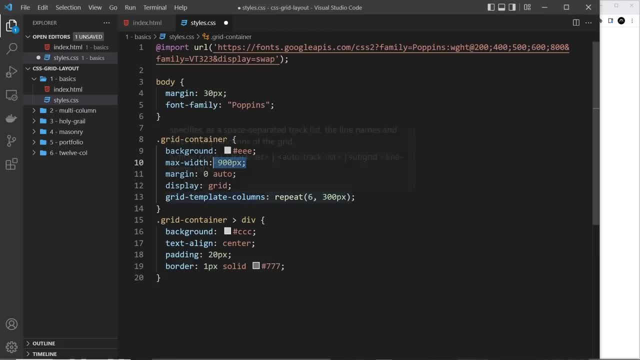 So we'd have to have 900 pixels divided by 6, So we could calculate that out and put it in here. all what we could do instead is use something called fractions, So I could say one fraction, So that means that we're gonna have essentially- let me just cut this- 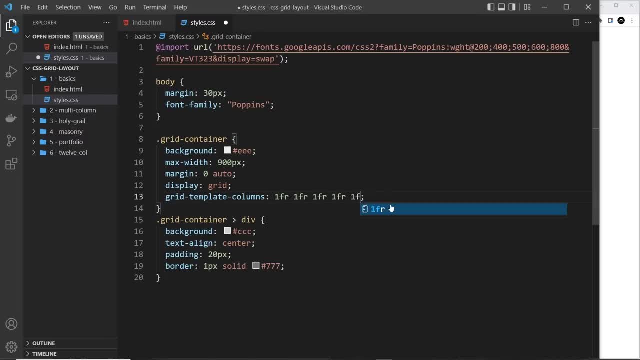 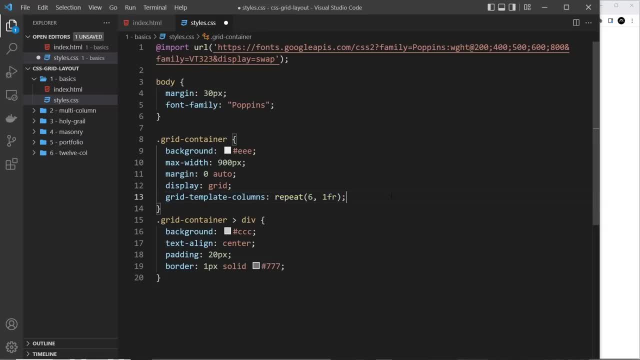 Okay, and this thing right here, when we use the repeat function, does exactly that as well. So now we're gonna have six columns, and each of those columns is an equal width, taking up the whole width, 900 pixels in total, and each item gets distributed in. 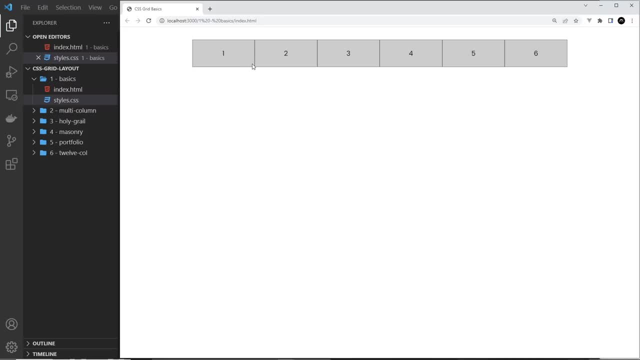 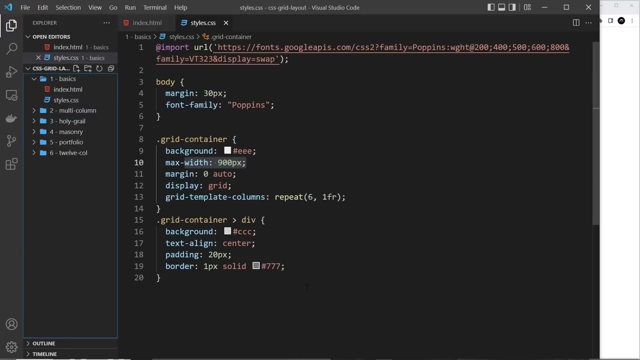 To one of those columns. All right, pretty cool, Yeah. Okay, so also we could add rows, but I'm going to show you that later on. in fact, for now, what I'm going to do is Start distributing these different grid items in different positions on the grid. 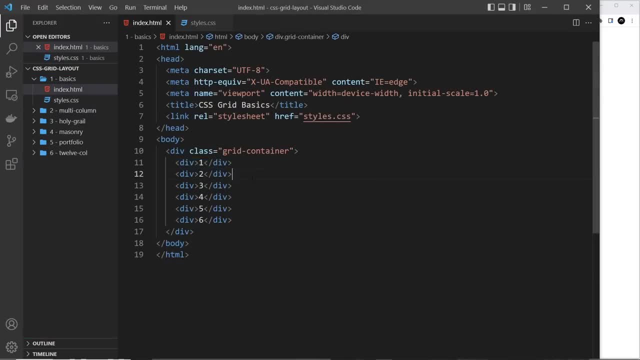 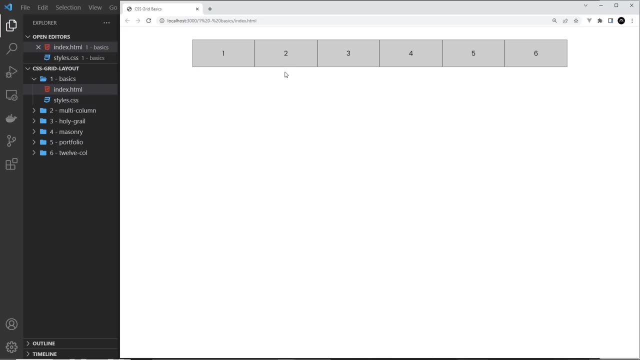 So, like I said, instead of these automatically being placed in the columns one after another, Like so, what we could do is say: okay, Well, the first one is going to take up three columns in width. The second one is going to take up two columns in width, the third one one. then on to the next row. 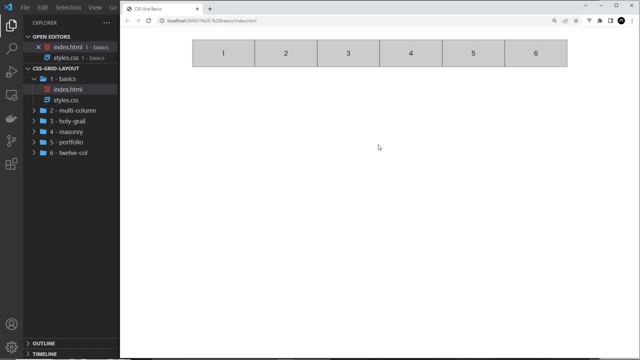 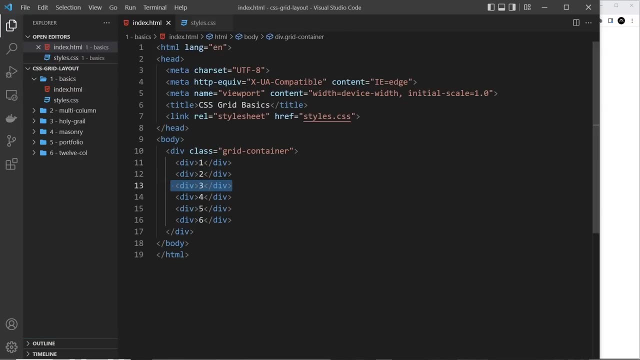 The first one is going to take up four, then two, etc. So we can do that kind of thing. so the way we're going to do this is by Stymie each one of these or targeting each one of these individually in the CSS, so we can assign each grid item. 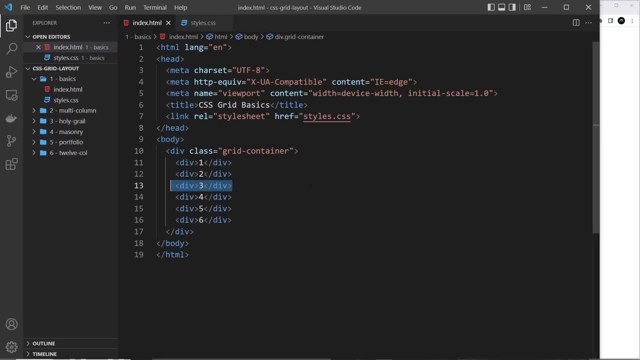 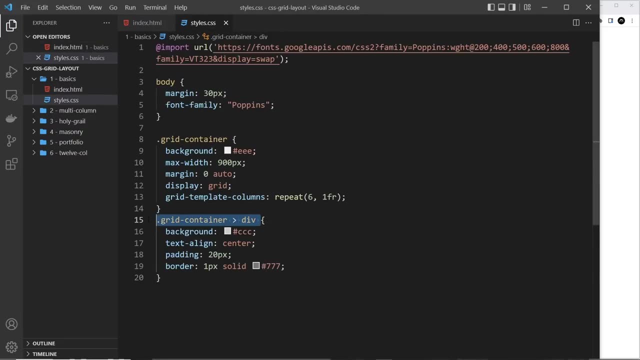 some kind of information to say where it's gonna sit on the grid. so We need to make selectors for each of these and to do that we're gonna be using nth child. so let me first of all copy that out and this selector and paste it down here, and then we're going to use nth child on this and this is: 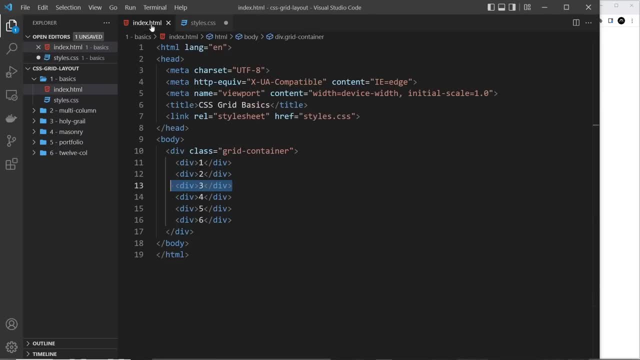 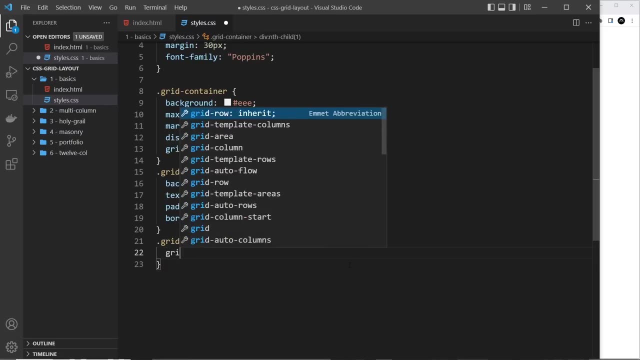 going to be the first one. so we're saying, grab the first child right here, the first div, and we're going to assign that somewhere on the grid. now what i'm going to do is use the grid hyphen column property to do this. this is how we manually assign an area on the grid, if you like, to a certain. 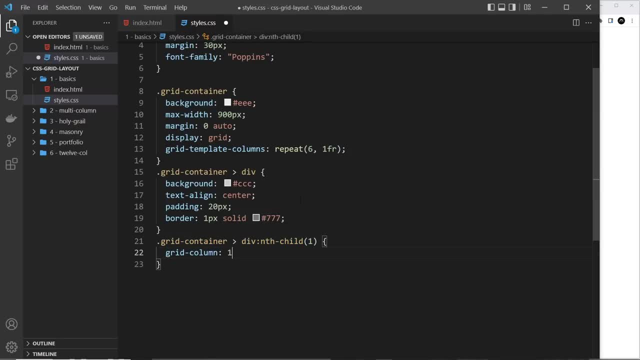 element. okay. so i'm going to say i want it to start at position one, at grid line one, if you like, over here. that's the starting position. and then i'm going to say forward, slash. and then after that we say either where we want it to end or how wide we want it to be. so, for example, if i want it, 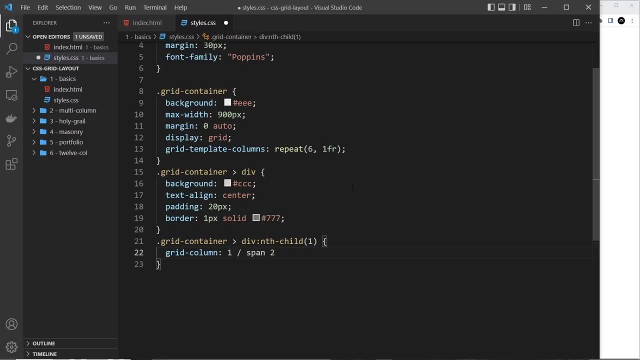 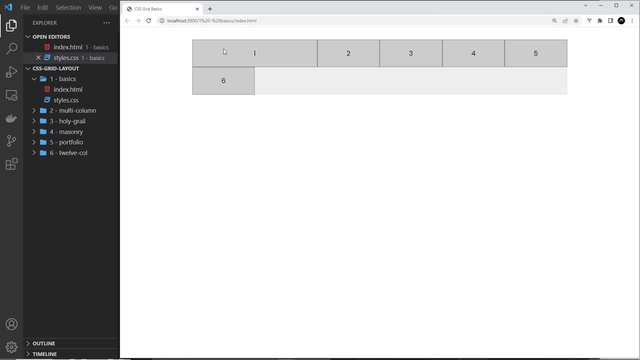 to be two columns in width. i could say span two and that means span this element two columns in width. so we start at this grid line one and we want it to be two columns in width. so this and this in total, all right. so let me save that and preview and now we can see that. 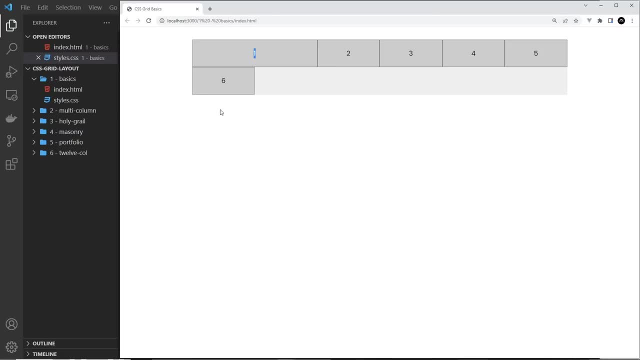 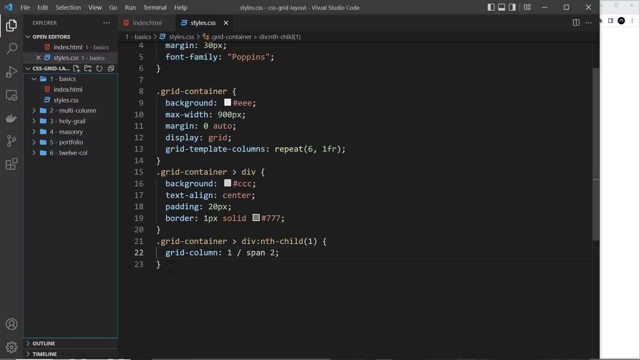 this one is two columns in width and it starts over here on the left and automatically. now it's budged this next grid item onto the next row, all right, so let's try something similar with the other grid items. so i'm going to copy this and paste it down here. i'm going to change this to: 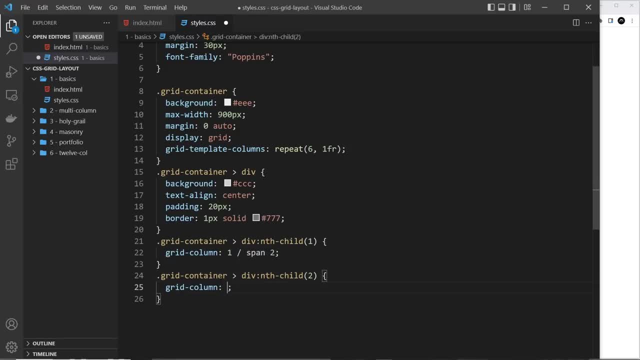 two, and let's delete this right here. so this time we're targeting the second child, this second grid item, and this we'll just say span three. now you'll notice, i've not added the first thing right here, so i've not added a start position, and when we don't add a start position, it just automatically starts at. 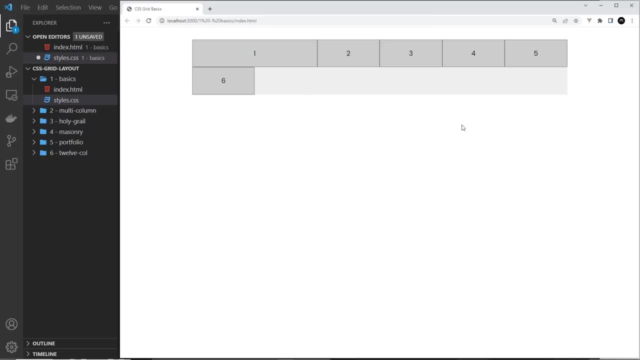 the next available position, so we don't need to say, okay, well, it's going to be not one, two, but start in position three. it automatically starts there because that's the next available position. so this will be the same as three forward slash span three. so let me show you this first of all. 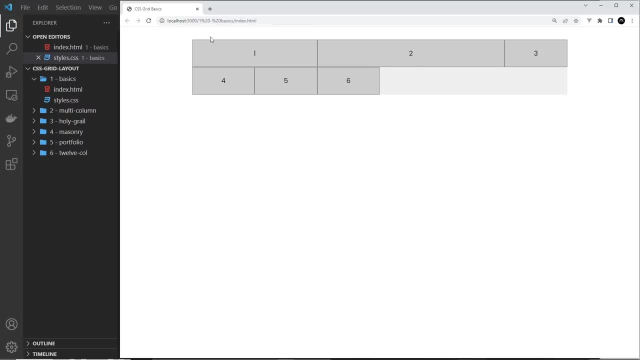 save and we can see it starts at grid line three: one, the second one is here, two and then three, so this spans three columns from that position. okay, so this is the same as this save it, and it's still going to be the same, and in fact the first one as well you could get. 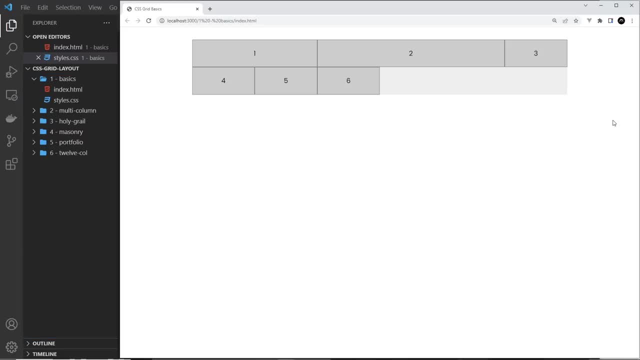 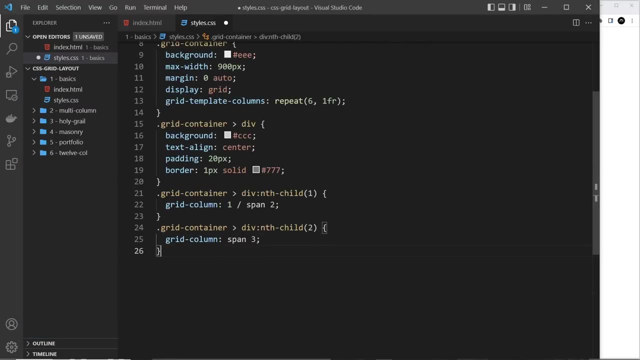 rid of the one, because it automatically starts at the first position. save it, and it's going to be exactly the same. but let's keep that in, just so we know what it is. okay. so let's move on to the next one. i'm going to paste this in again and say: third child this time, and 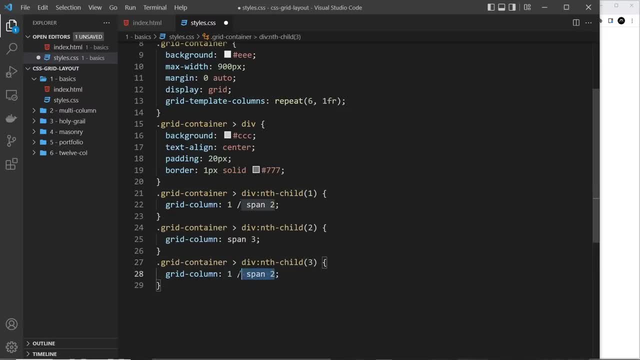 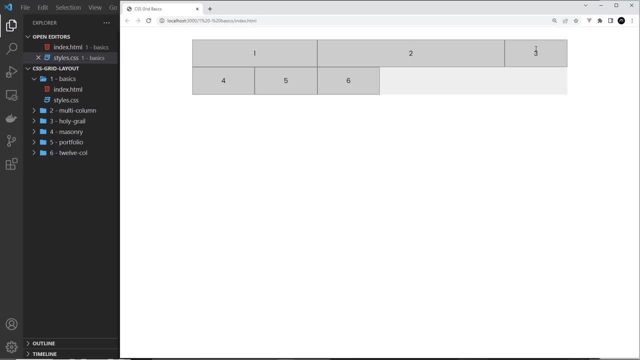 for this one, i will say: grid hyphen column is going to just span one. well, it automatically spans one anyway. okay, that's the default behavior. so if i didn't have this, then it would do exactly the same. so it automatically spans one column in width anyway. but let's be explicit, just so we can. 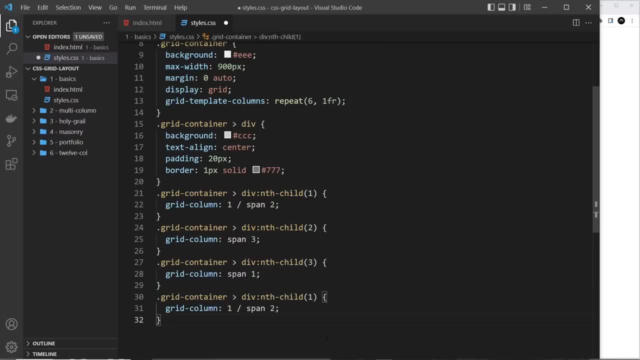 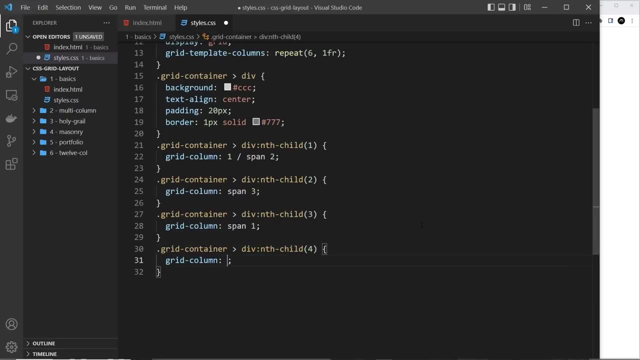 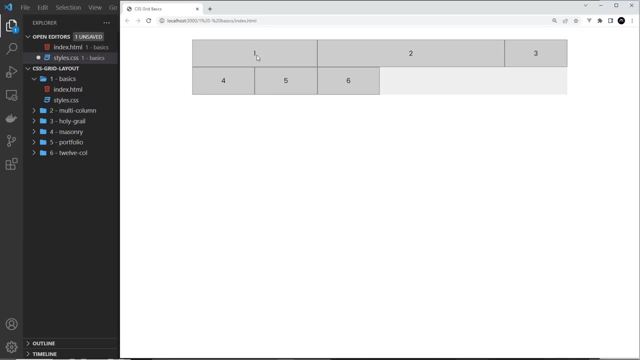 style each one. i'm going to move on and we'll do the fourth one. so change this to four. and this time the grid hyphen column will say: is going to start at line two. so that's one. two, so it starts here on this row. okay, this time that's where it's going to start, and then forward slash to say how. 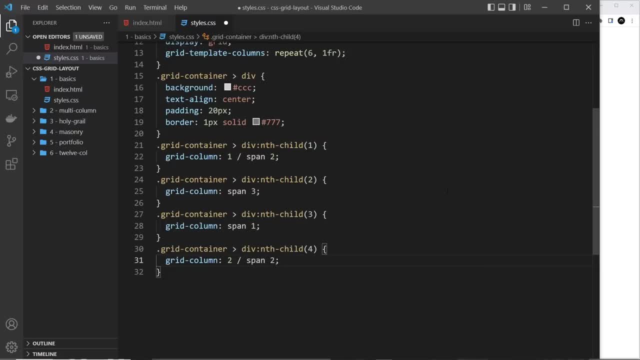 wide we want it to be, so i could say span two columns or something like that if i wanted to. but also over here we could just specify the end grid line. so what grid line we want this element to go up to. so i could say here six, and then it's going. 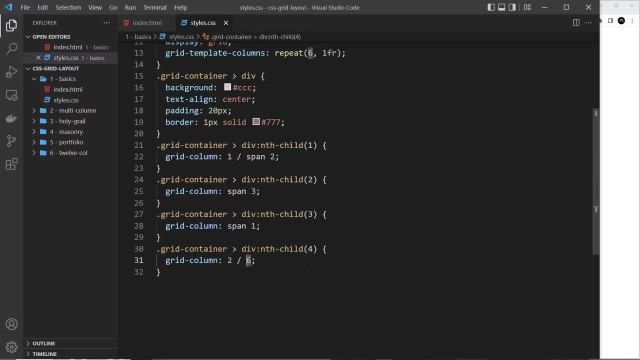 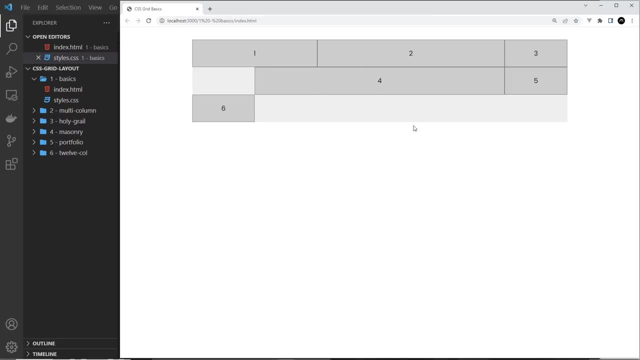 to span from the second grid line all the way to the sixth grid line. so let's save that and we can see. so this is the first one: two, three, four, five and six. so it goes all the way up to the sixth grid line, or column grid line right here. okay, 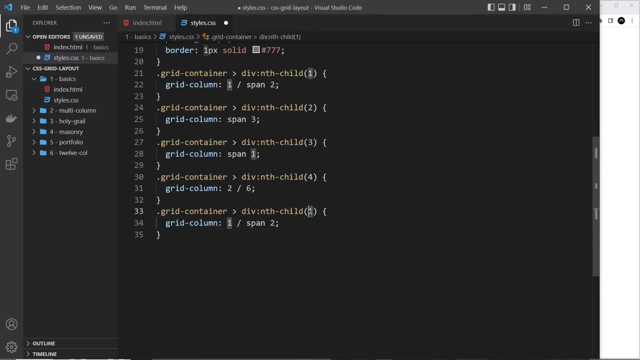 all right, let's go on to the fifth one. so change this to five now and let's delete this, and what we'll say for this one is: just span three columns in width. now at the minute it's right here so it sits on the same row. but if we add span three, we're saying we want it to be three columns. 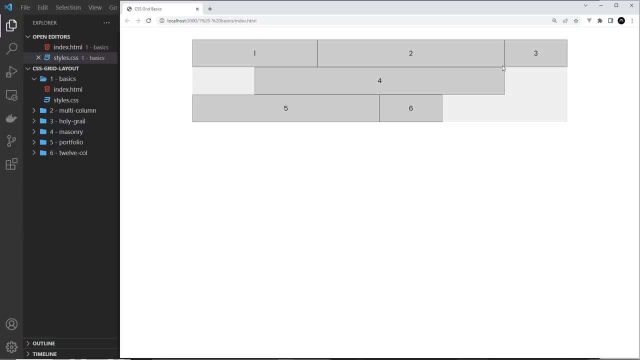 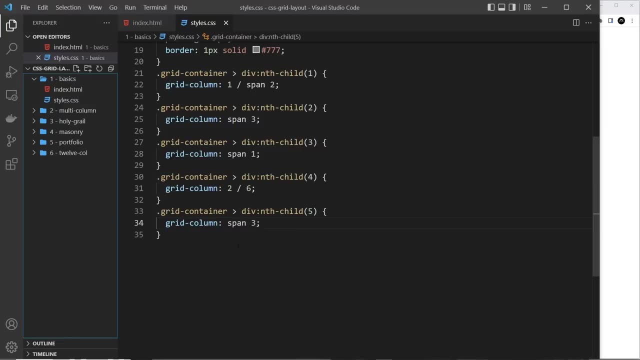 in width. now that doesn't exist, that amount of space on the current row right here, so it goes to the next row down right here and we have three columns in width. and then let's do the last one: paste this in, change it to six, get rid of this, and again we'll say span three, like so, save it, and 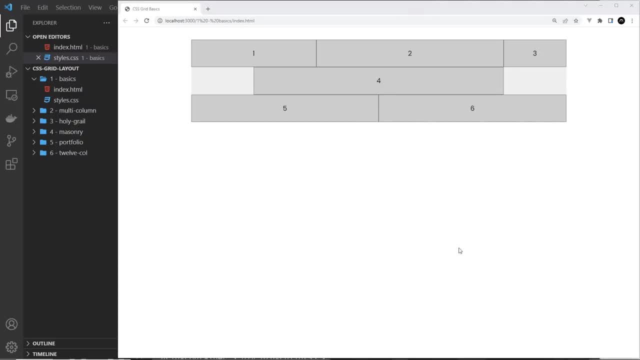 we can see it takes up the other three columns in width on that row. okay, so as we're distributing these grid items onto the grid, notice that when we run out of space on a particular row, the next grid item automatically shifts to the next row. okay, that's how we get multiple rows in the grid. 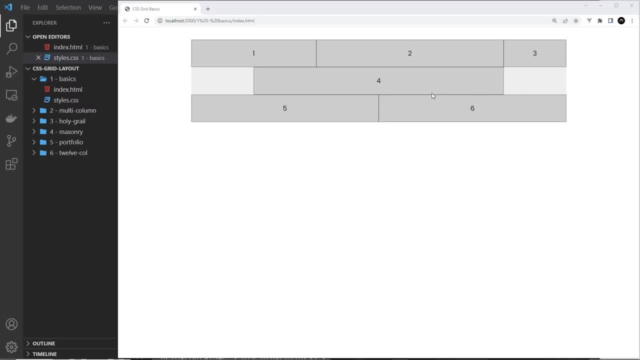 now also notice that the row height is specified, or rather dictated, by the width of the grid, so by the height of the grid items themselves, these things. now we have a height on these because we gave them padding before and at the minute all of these rows are the same height. but what i can do? 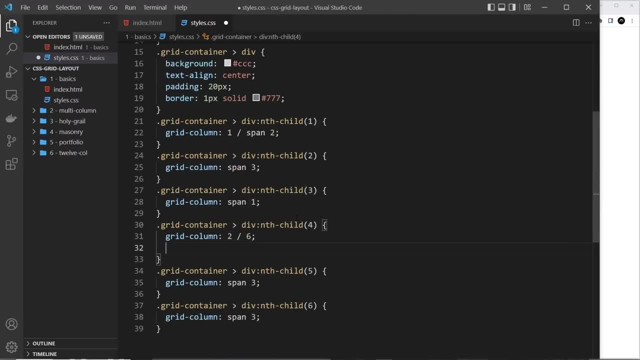 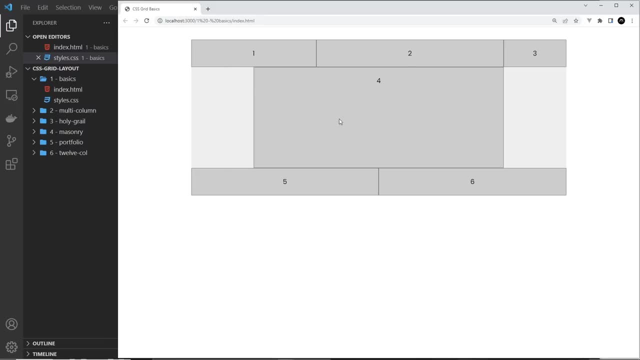 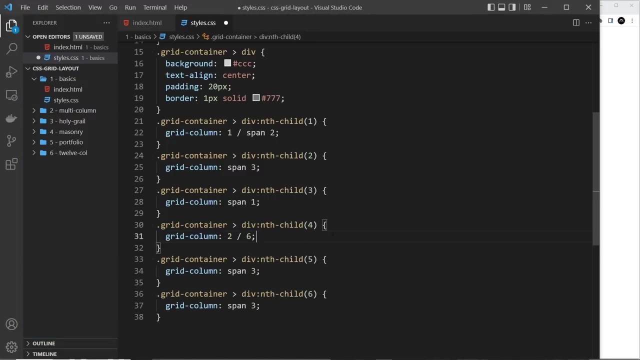 is come to the fourth one over here and give this a height of 200 pixels, and if we check this out, we're going to notice that this row height now is 200 pixels, dictated by the height of the content inside it. okay, now we can also specify the row height if we go up to the container up here and 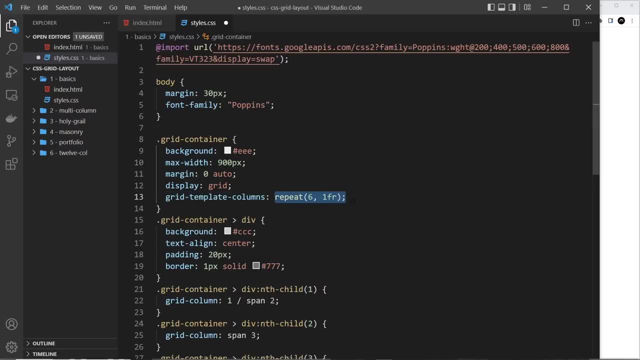 we have grid template columns to specify the width of columns in the grid. we can manually specify the height of rows in the grid by using grid template hyphen rows like so: now we have three rows in our grid at the minute, so what i want to do is three difference, or they could be the same. 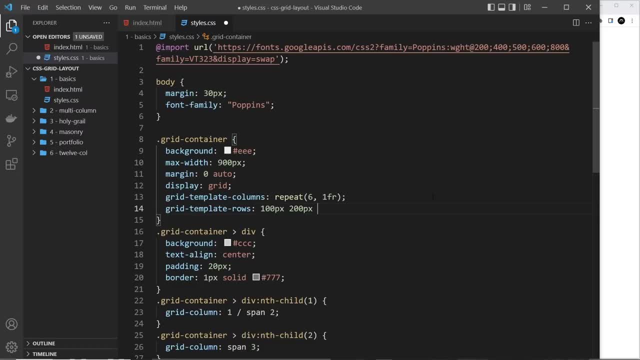 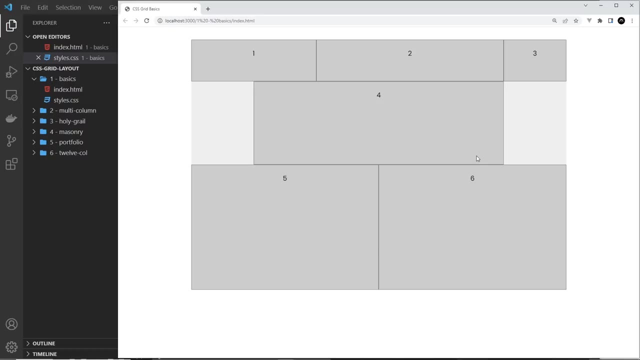 values right here. so i could say 100 pixels, 200 pixels and 300 pixels and that means the first row is going to be 100 pixels in height, the second row 200 pixels and the third one 300 pixels. so if i save this, we can see that right here and notice also that when we manually set the height, 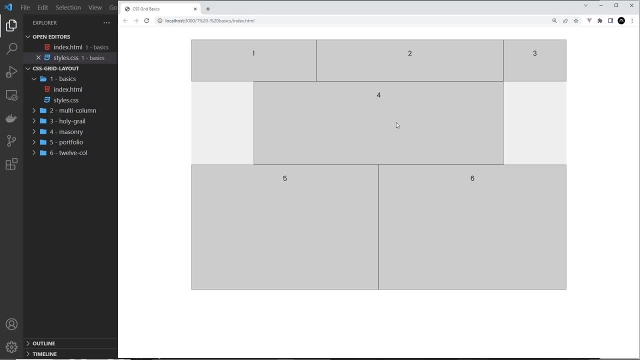 of the rows. the content inside those rows stretches to match the height of the row, so it takes up the full height every time, and that's the default behavior of grid items in a grid in the rows. okay, now we can override that behavior, and i'm going to show you how to do that later on, but for 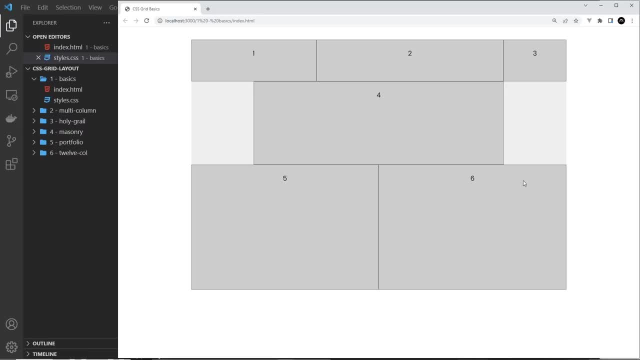 now i also want to show you another property to add a gap to the grid. so you know, like we talked about this before, which was how we space the columns and the rows out. well, we do that using a gap property. so i could come over here and say the gap is going to be 10 pixels, like so. 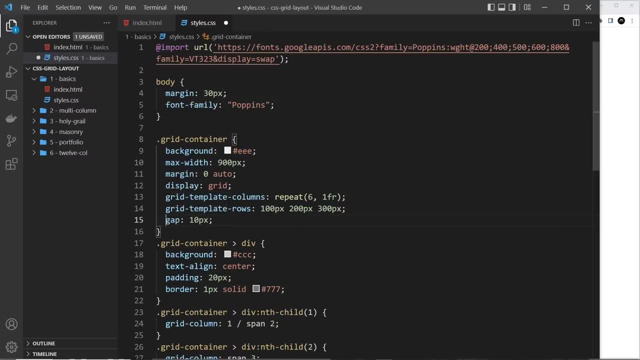 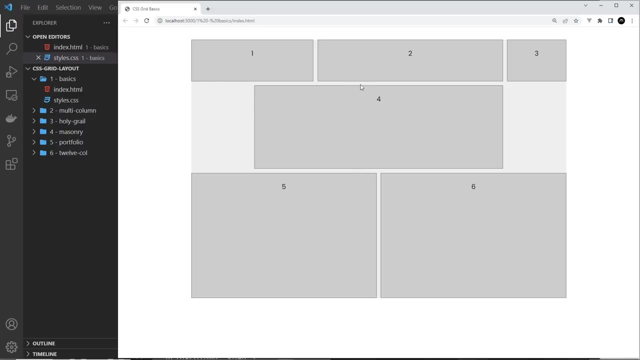 you might also see grid hyphen gap as well, but i'm going to leave it as gap: 10 pixels, and that means we have a 10 pixel gap between every column and every row. okay, so if i save this, we can now see this stuff is spaced out a little bit, so between every row we have this 12, or rather 10 pixel. 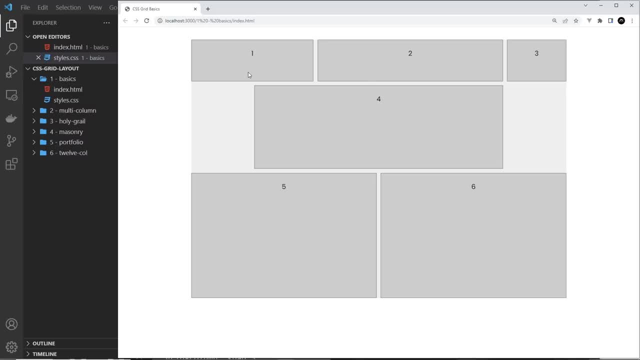 gap, and between every column we have it as well. now you might be thinking: well, there's no gap right here. there's none here inside these rows, where the elements are, and that's because we have the elements sitting over them. so where an element takes up, say, three columns in width, 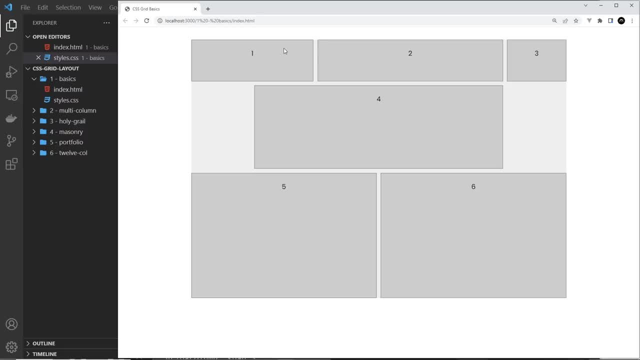 you obviously don't see the gap underneath that element. it kind of spans the entire width of those three columns, but where the next column starts after that with a new element, we do see a gap. okay, cool. now i want to show you another thing which is pretty cool. 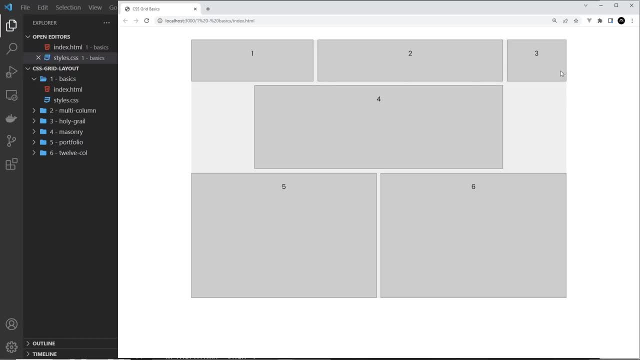 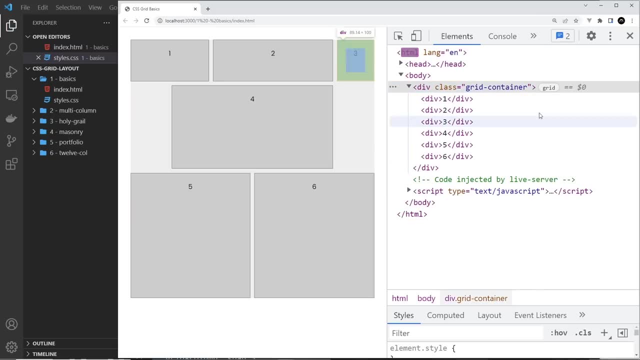 and that is a tool in chrome, but you can also get this in firefox as well. if i right click and inspect a grid and then go over here, what i'm going to do is just refresh the page. we can see this grid bubble right here, and if i click on this, then we can actually see an overlay of the grid. 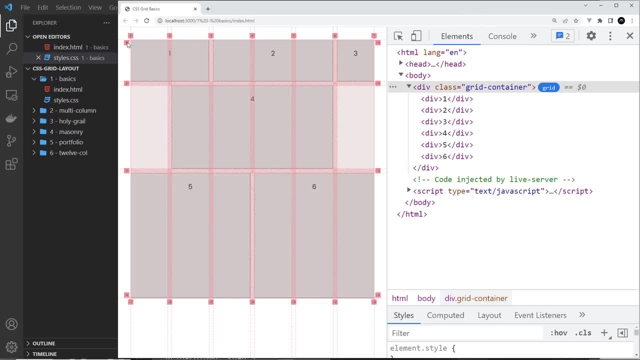 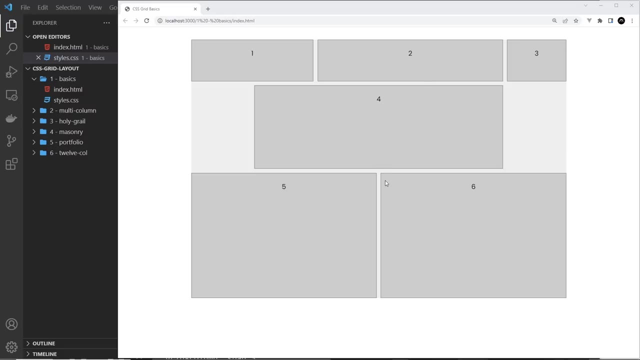 over here so we can see the grid lines for the columns and also for the rows, we can see the rows themselves and we can see the gutters or the gaps as well. so that's pretty nice. it's nice to have in the browser. cool, all right. so the last things i want to show you is how to align items and 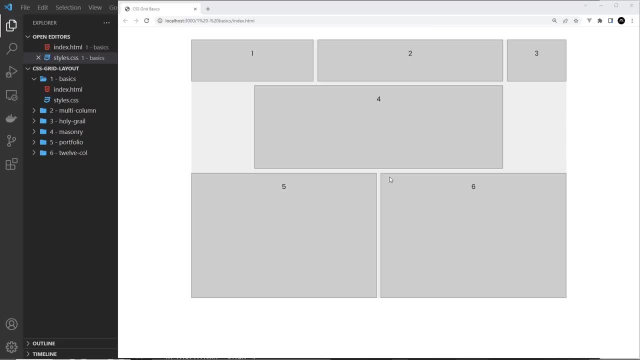 justify items. so when we talk about justifying items, we're talking about how they're justified going across the columns, and when we talk about aligning grid items, we're talking about how they're aligning going vertically down the rows. okay, so remember how i said the 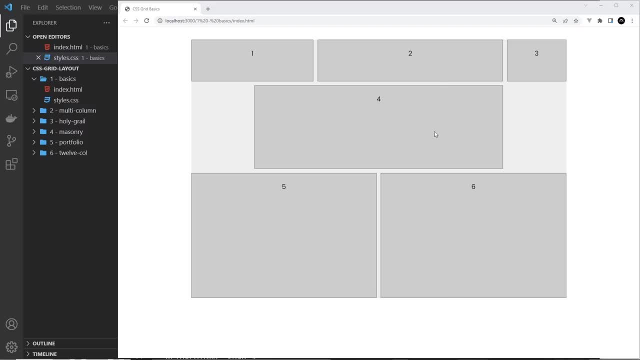 default behavior of these grid items is to stretch the height of the rows, but not also that to The width of the columns they're taking up as well. Well, we can override that behavior. So I'm going to come over to the grid container and I can use a property called justify. 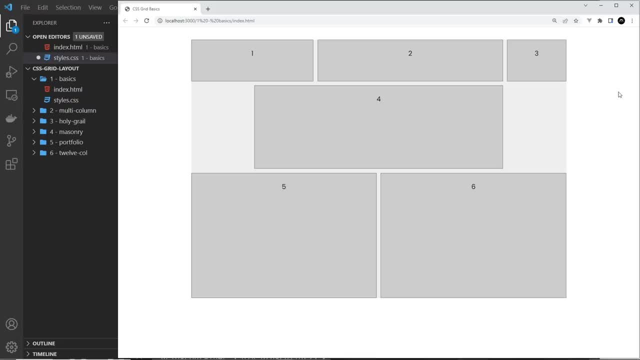 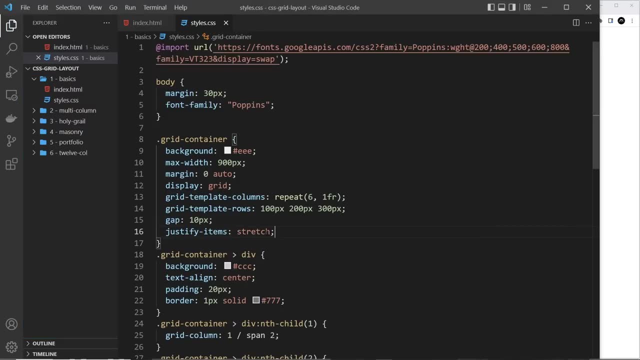 Items. I remember I said justify is when we're talking about how items are justified going across. now, The default value, like I said before, is stretch, meaning each item, each grid item Stretches to take up the full width of the columns It's been assigned. but you can override this to be a different value. 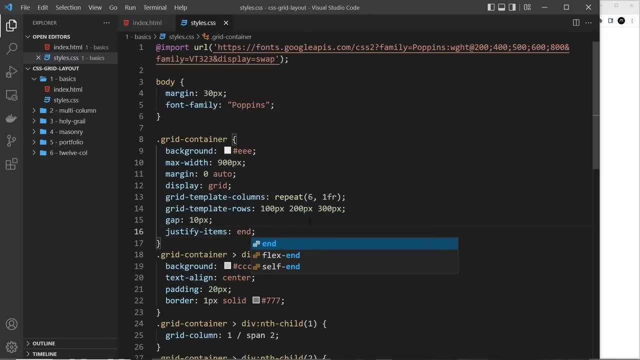 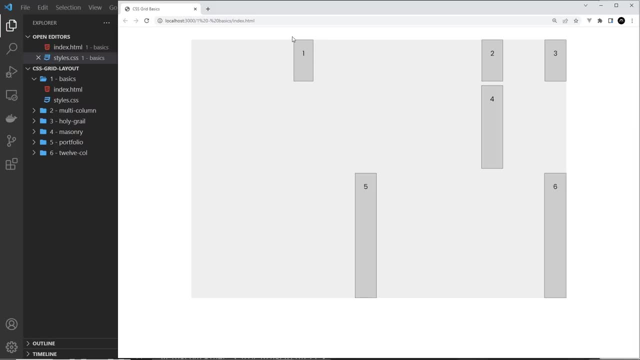 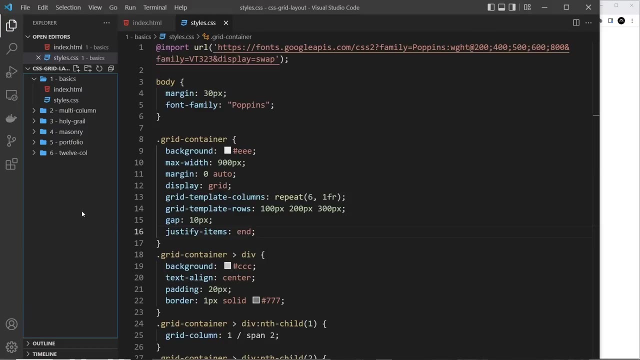 So we could have instead end- and if I save this, you're going to notice each of these now Doesn't stretch to take up the full width of the columns They've been assigned, but instead they go to the end of the columns They've been assigned. So this is the very end of the first two columns, because the first one we span it to right. 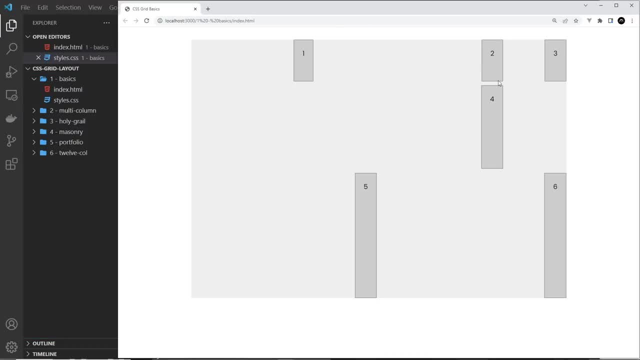 So this is the end bit of the first two columns. this is the end bit of the next three, the end bit of the third one, Etc. Okay, So now they're all sitting at the end of the allocated columns Going across. we could change this to be start, if we want as well. 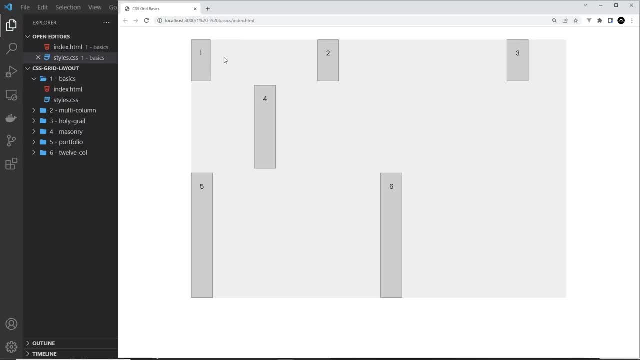 like so, and that moves them to the start of their allotted columns. and This could also be Center, and it moves them to the center of the allocated columns. All right, So I'm going to change this back to stretch, which is the default behavior to stretch across the whole. 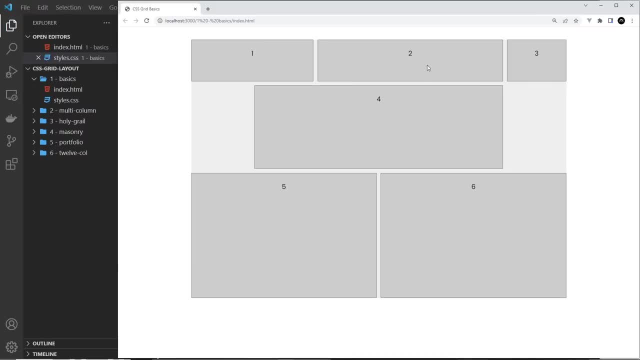 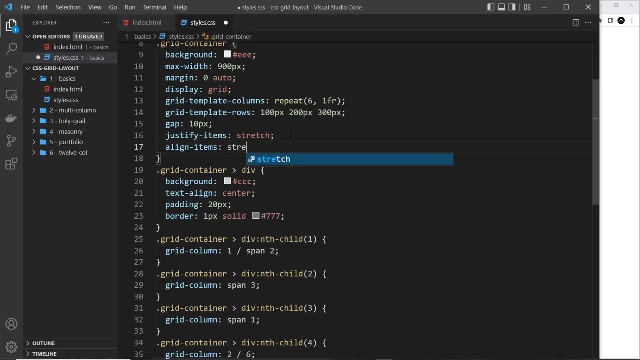 Columns that they've been allocated, and we can also do that. We're the same thing up and down using a line items Like: so we're going to use the same properties. So the default is stretch, which is what at the minute, but I can change this to start. 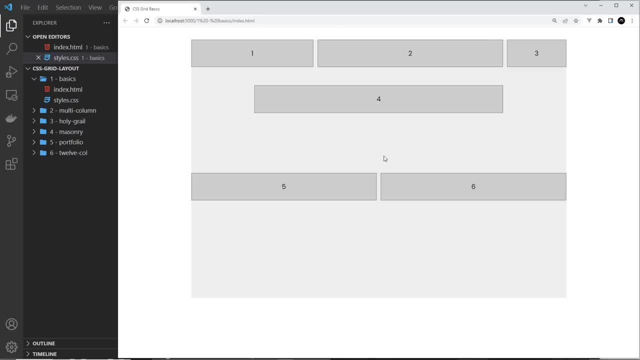 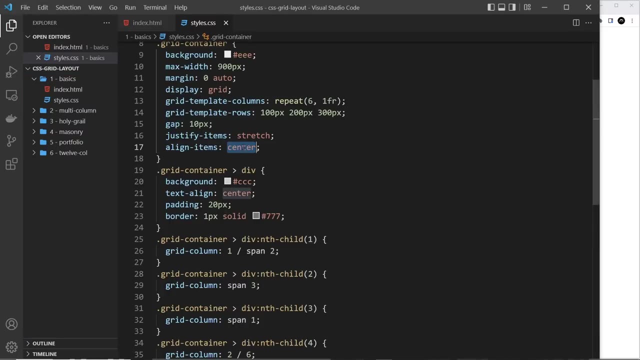 and if I save that, then they're gonna sit at the top of each row that they've been allocated, and If we change this to end, then they're gonna sit at the bottom, and if we change it to Center, They'll sit in the middle, like so. so what I'm gonna do is 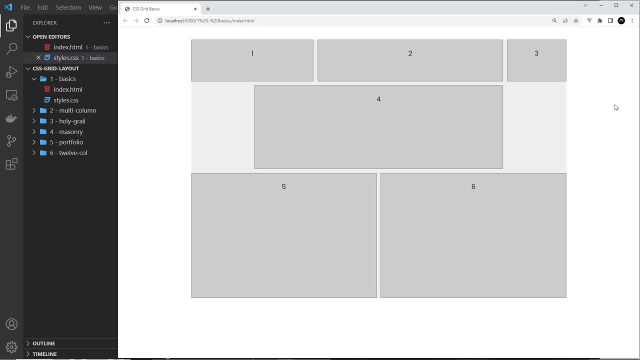 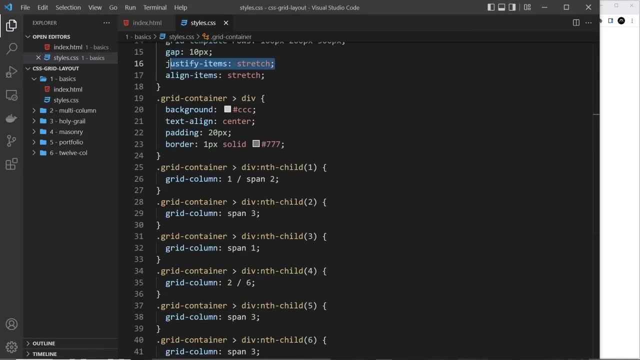 Keep this as stretch as well to be the default. now You might want it to be that you don't style all of them and you just want to override one of the grid items. So, for example, I could come to the fourth one and I might want to align. 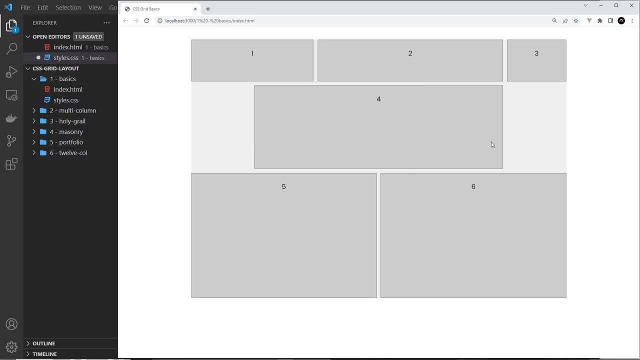 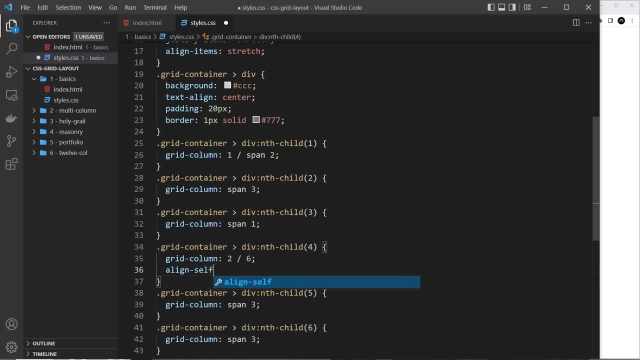 This, this particular grid item, to the end. so it just sits down here at the bottom of the row, and I can do that by seeing a line, because we're going in A vertical direction, and then self so align items and justify items up here. I'm gonna do the same thing right here on the grid container. 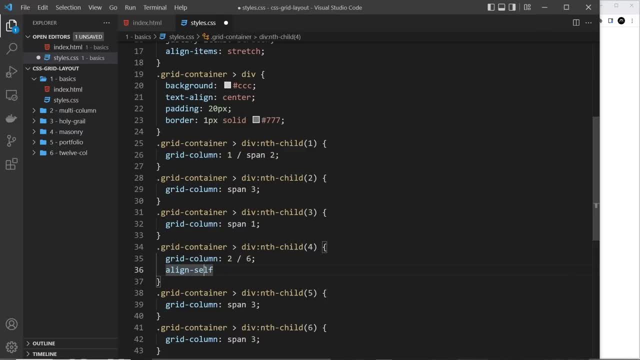 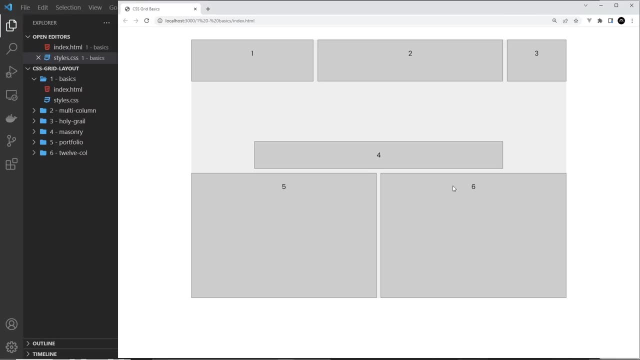 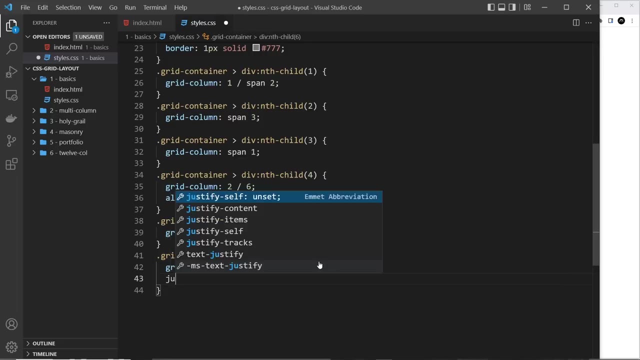 But when we're overriding individual grid items, we say align self, or if we're using justify, justify self, So Colan, and then this is going to be end Like so, and now it should sit at the bottom of the row, Awesome. So I'm also going to do this with the last one. 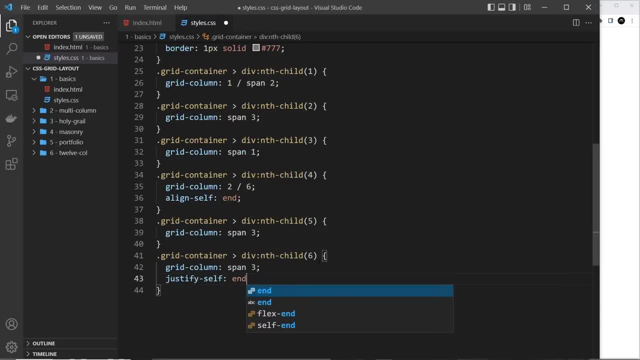 I'll come over here this time. I'll say justify Self and we'll say end for this as well. So end, it's gonna sit over here. Justify means going across равно. i'm also going to use align self as well, and that's going to be start this time. so it should. 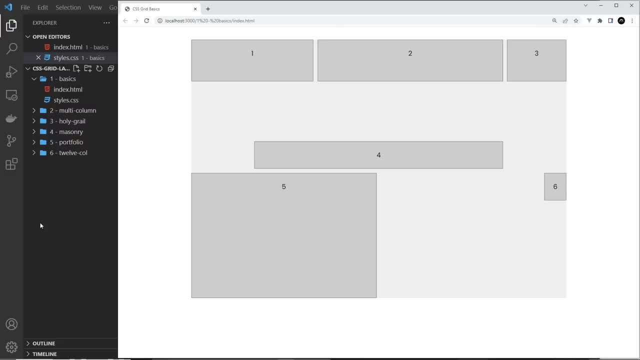 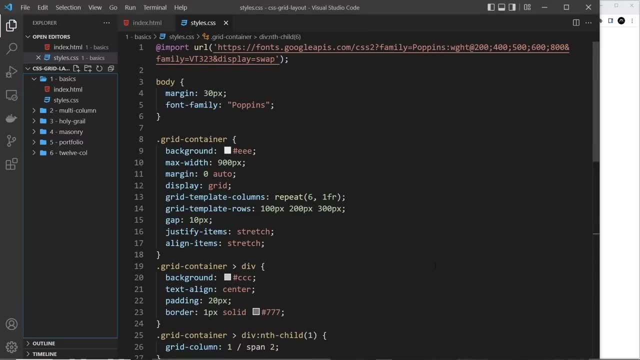 sit at the top right here, awesome. so there we go, my friends. i think we've covered enough of the basics of css grid now and i think you should know enough to tackle the projects that we're going to create in the rest of this series. so in the next lesson we're going to move on and start our first. 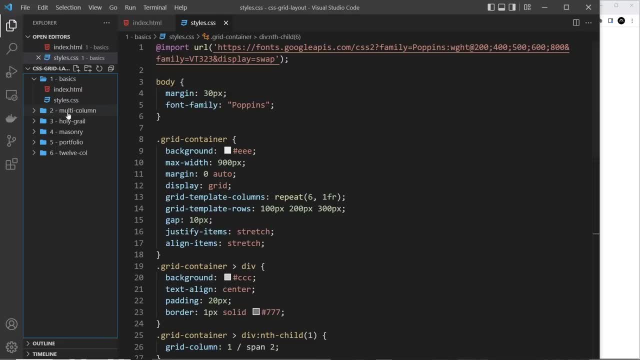 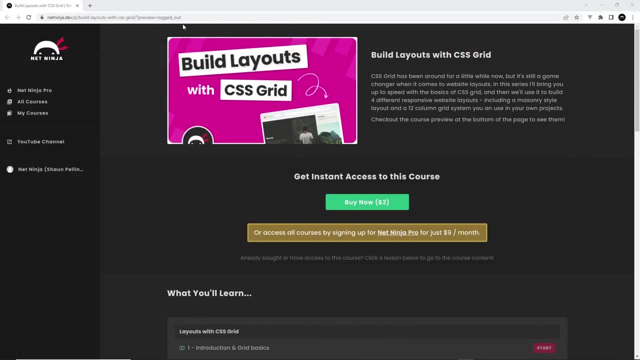 project, which is the multi column layout- this one right here, by the way. if you want to watch this entire course now without youtube adverts, you can do. it's all up on the net ninja website, net ninja dot dev. you can buy the course for two dollars to get instant access to all of it, or you can sign up. 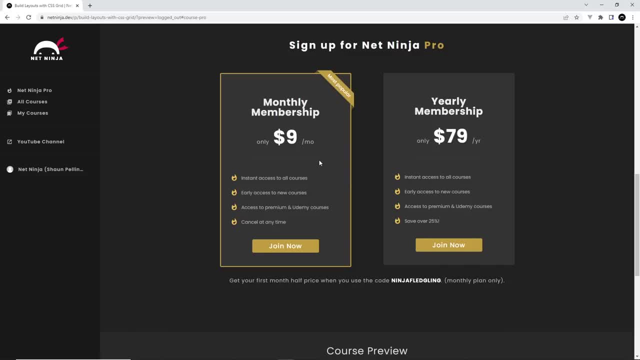 to net ninja pro and get instant access to all of my courses without adverts, as well as premium courses not found on youtube, including my udemy ones. that's nine dollars a month, and you can get your first month half price when you use this promo code right here. so i'm going to leave this. 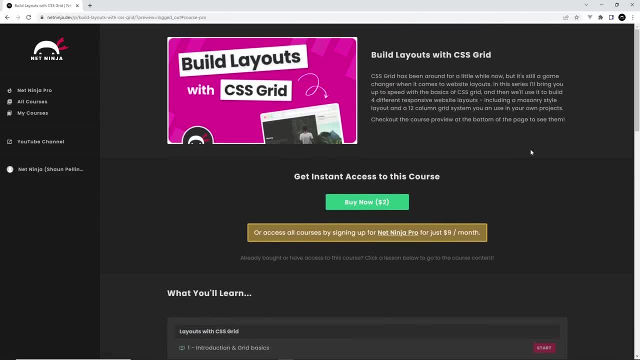 link down below in the video description for you to sign up, and i really hope you enjoy this series and please do not forget to share, subscribe and like the videos. that really helps a lot and i'm going to see you in the very next lesson.